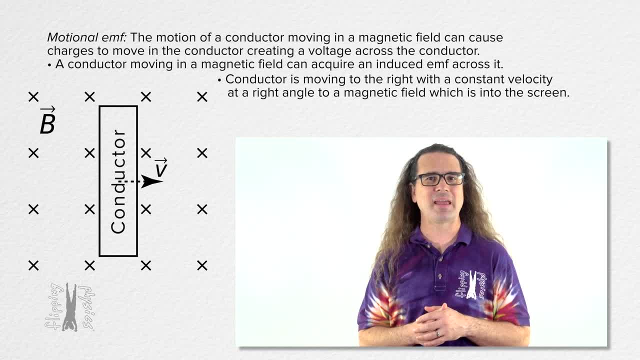 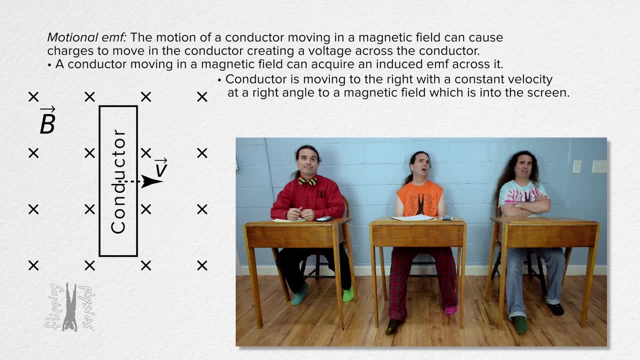 right with a constant velocity, at a right angle to the magnetic field which is into the screen. Sure, Objects can just fly at constant velocities through magnetic fields. That makes sense. It's an airplane. He's showing a simplified view, Yeah. 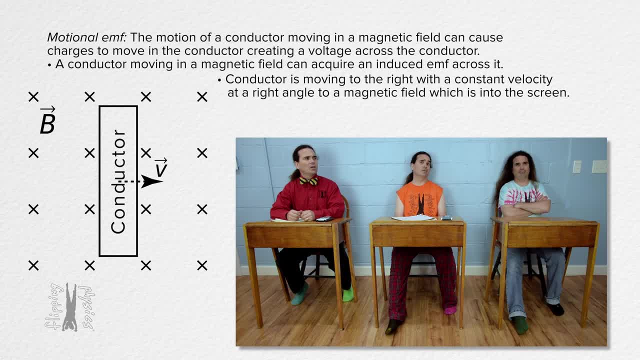 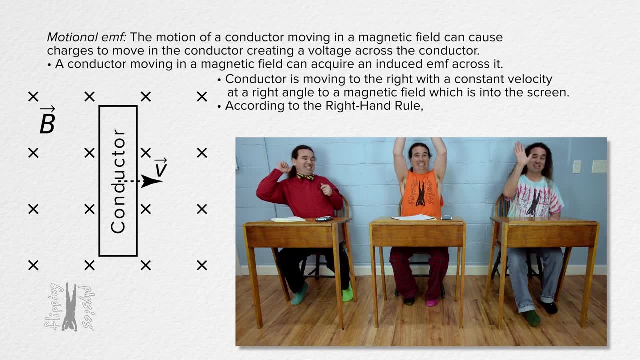 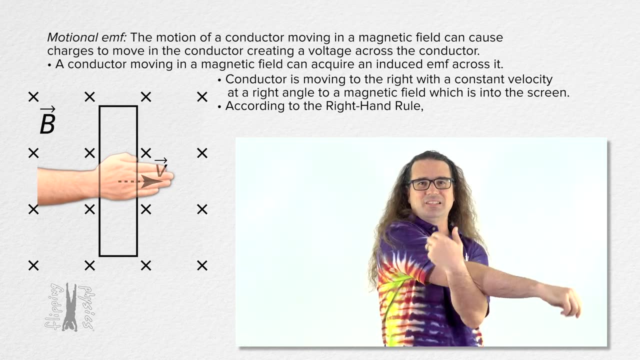 It's a version of an airplane wing flying through the Earth's magnetic field. Right, Sorry, Yeah, Yep. According to the right-hand rule… Don't be too cool, Limber up And find your right hand. According to the right-hand rule, fingers point to the right with the velocity of the charges. 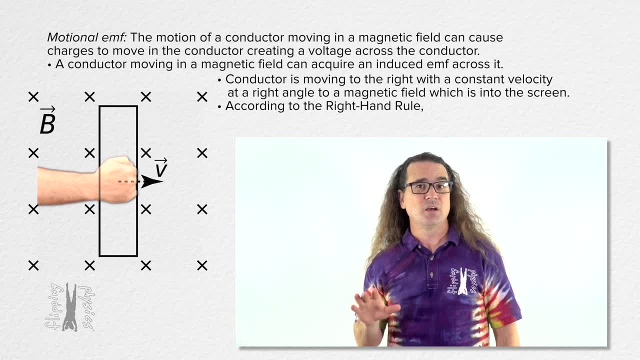 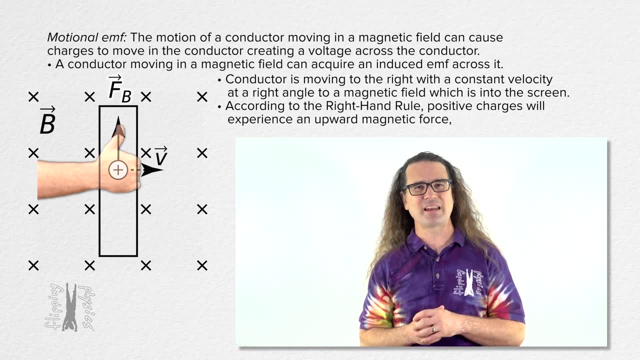 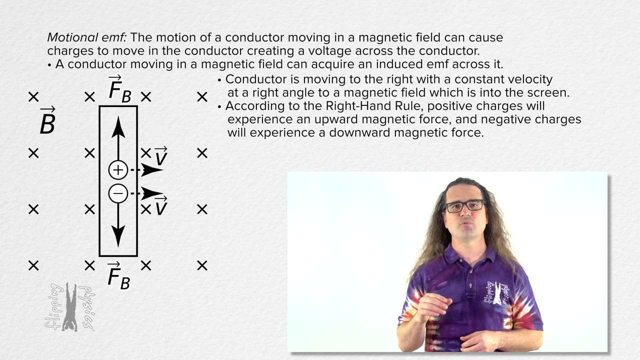 curl fingers into the screen with the magnetic field thumb points upward toward the top of the screen. That means positive charges will experience an upward magnetic force and negative charges will experience a downward magnetic force. This will cause the charges to move, with the final result being that there will be a net positive charge on the top end of the 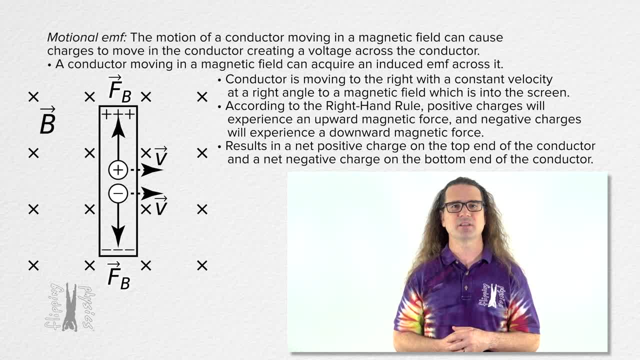 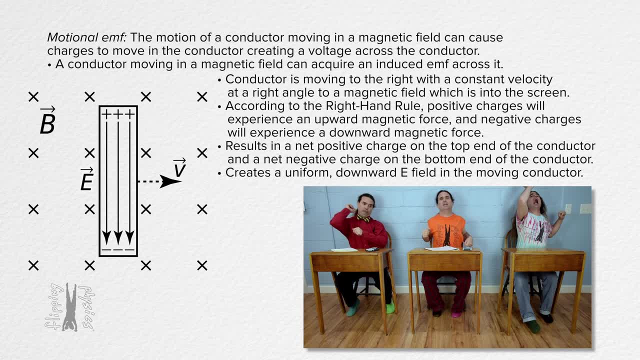 conductor and a net negative charge on the bottom end of the conductor. This arrangement of charges creates a uniform downward electric field in the moving conductor. I thought only electrons or negative charge carriers moved in conductors. right, That's what makes them conductors: They have lots. 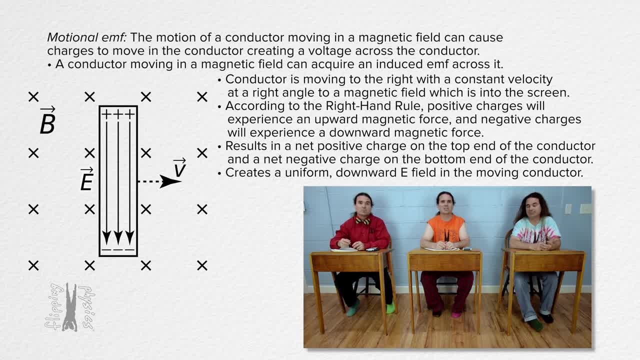 of free electrons which are able to easily move around in the conductor. That's why he used the phrase net charge when referring to the net charge on each end of the conductor. The positive end must have lost electrons to create a net positive charge there, and the negative end must have gained electrons to create a net negative charge there. He just 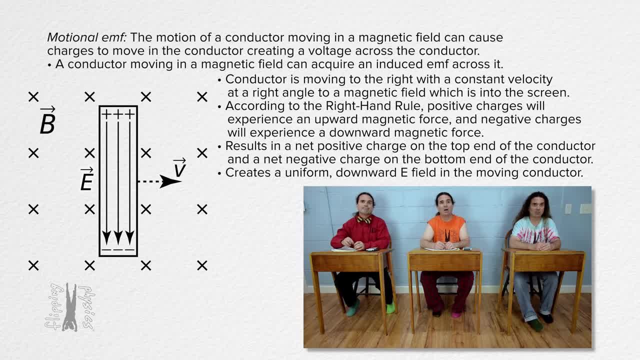 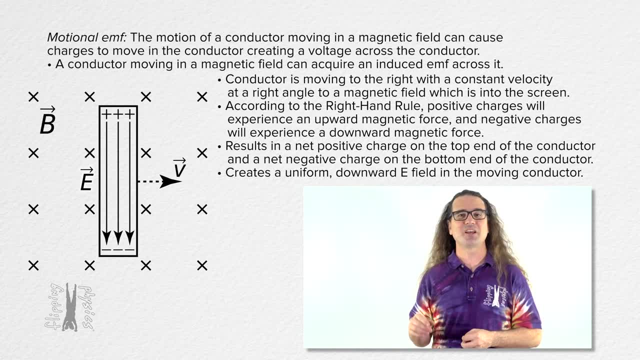 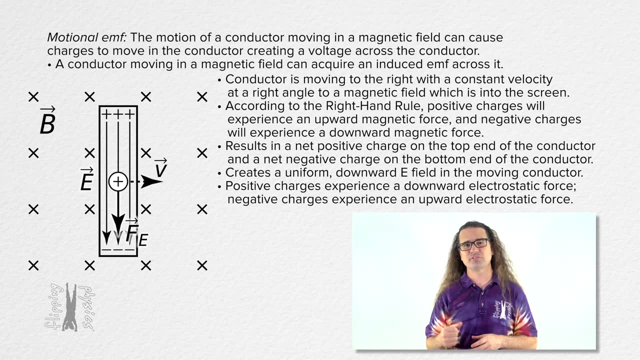 likes to talk about what happens to both positive and negative charges in conductors. to be complete, or something, Right, Mr P? Sure Yeah, As a result of the downward electric field in the conductor, positive charges will experience a downward electrostatic force and negative charges will experience an upward electrostatic force. 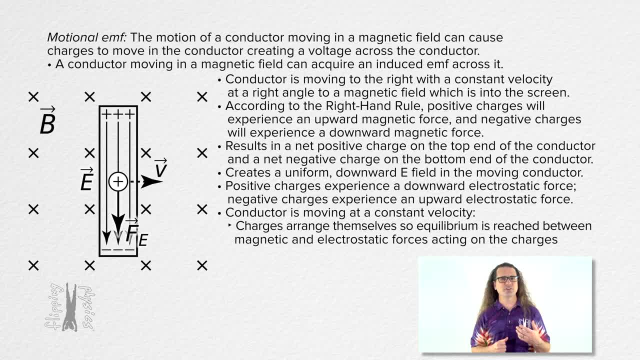 Because the conductor is moving at a constant velocity, the charges will arrange themselves such that equilibrium is reached between the magnetic and electrostatic forces acting on the charges, such that the electric field has a constant magnitude and the charges in the conductor are moving with a constant velocity to the right. 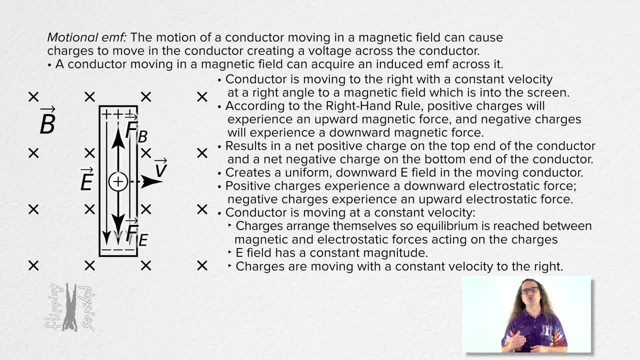 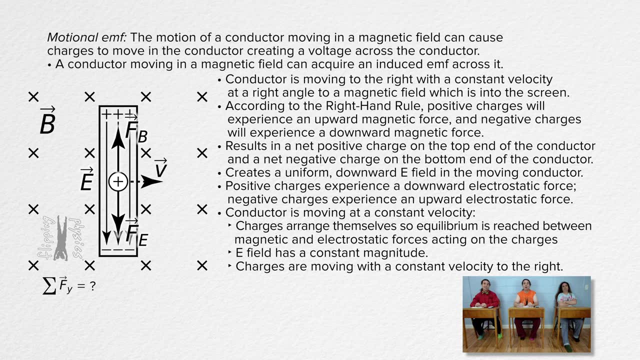 When it reaches equilibrium, there is no vertical motion of the electric charges. Billy, please sum the forces in the y-direction on a positive charge in the conductor which is moving to the right at a constant velocity, Absolutely Well, the net force in the y-direction acting on a positive charge. 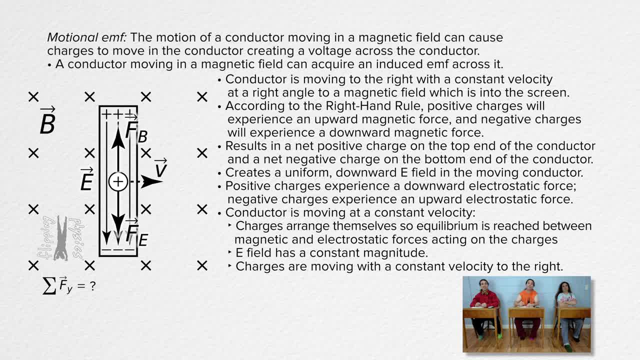 in the conductor, which is moving to the right at a constant velocity, equals the magnetic force minus the electric force, which equals mass times. acceleration in the y-direction: Because the positive charge is moving to the right at a constant velocity, the acceleration of the charge in the y-direction equals zero. 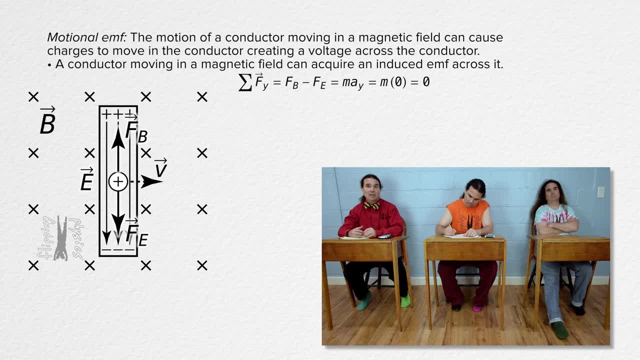 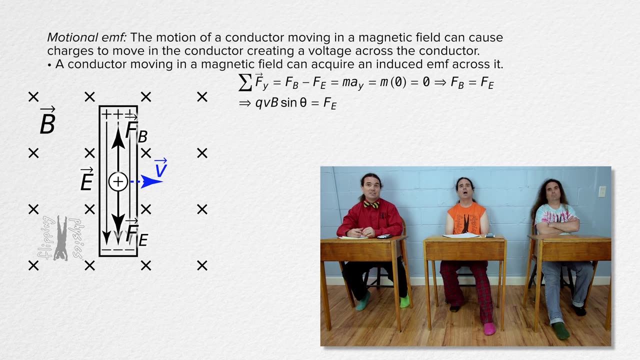 That means the magnitudes of the magnetic force and the electric force are equal. The equation for the magnetic force is: charge times, velocity times, magnetic field times, the sine of the angle between the directions of the velocity of the charge and the magnetic field. Velocity is to the right and the magnetic field is into the screen. 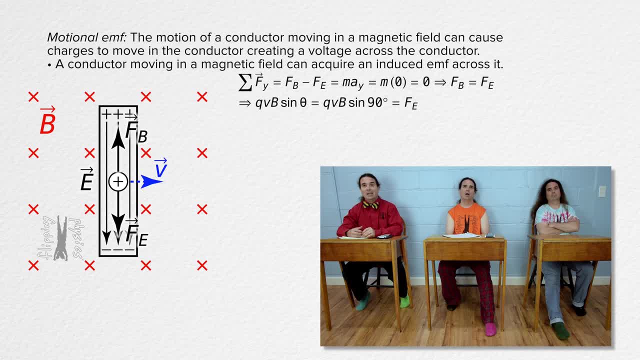 The angle between those two directions is 90 degrees. The sine of 90 degrees equals 1.. That's the left-hand side of the equation. On the right-hand side of the equation, oh, electric force equals charge times, electric field. So everybody brought charge to the party. 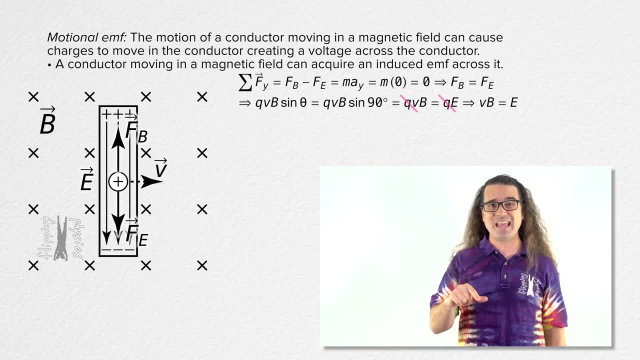 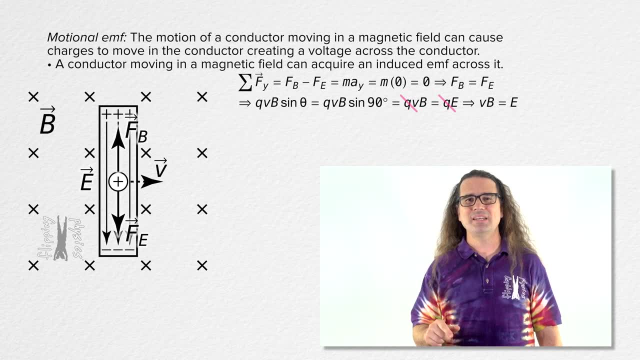 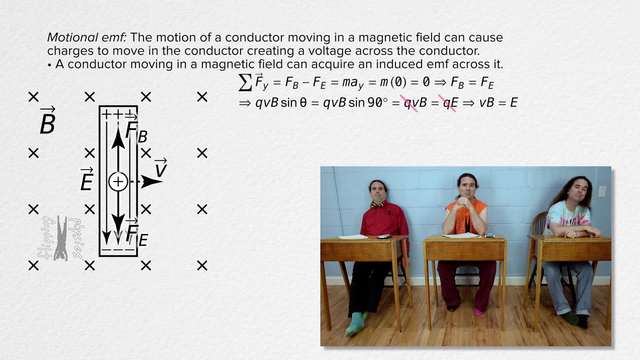 Please realize that if you summed the forces on a negative charge, moving in the conductor instead, you will arrive at the same equation we have here. And Bobby, what is the equation for the voltage across a uniform electric field? The equation for the voltage across a uniform electric field. 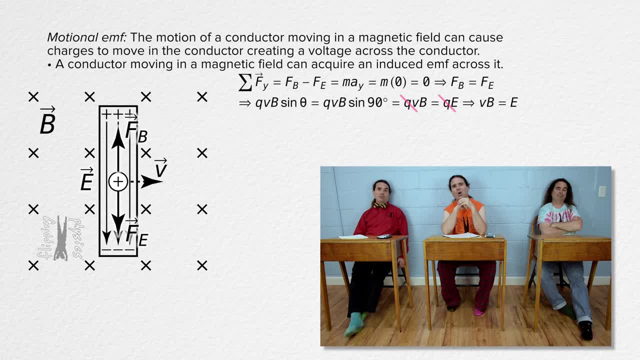 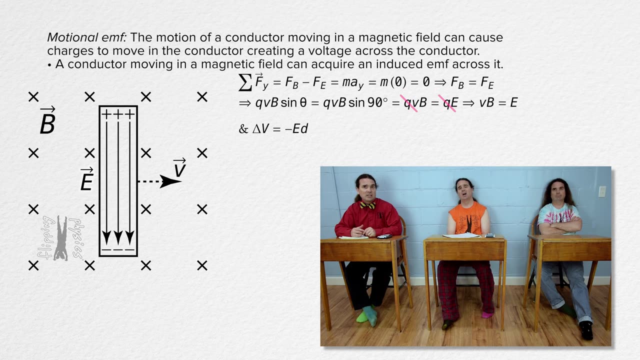 Remember we derived the equation for the electric potential difference between two parallel plates, And two parallel plates of opposite charge create a uniform electric field, which is basically what we have here, Kind of It's been…. …a, while The voltage across a uniform electric field equals the negative of the electric field times d. 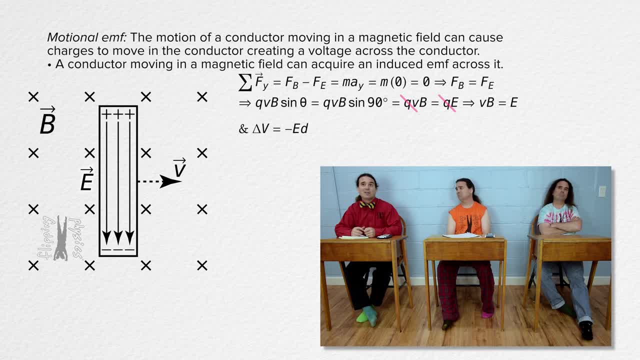 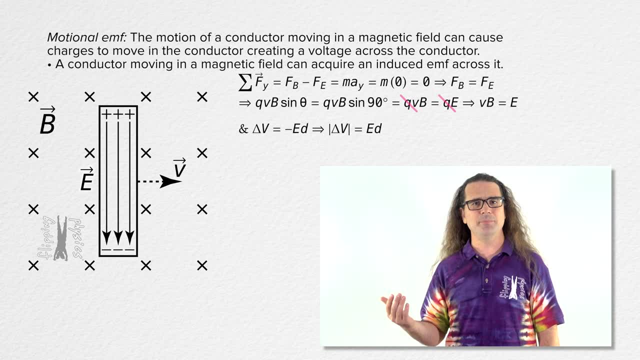 the distance between the two plates. Sure, That looks familiar. Thank you, Billy. We have already determined everything about directions here, so let's use the absolute value of the voltage And let's identify the length of the conductor to be capital L. 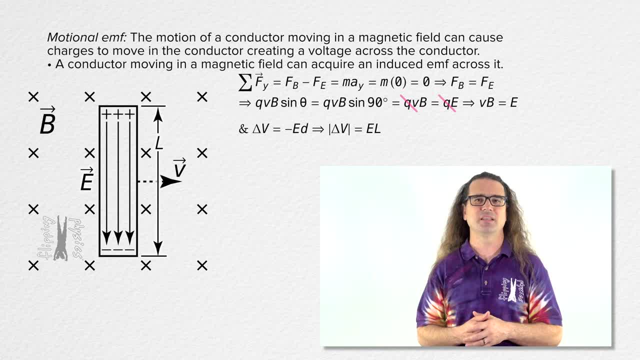 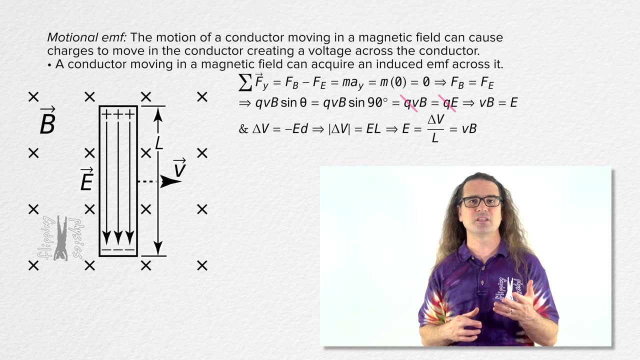 which is also the distance d, the length of the electric field in the conductor. We now know the electric field equals the voltage across the electric field across the conductor divided by the length of the conductor, And that also equals the velocity of the conductor times the magnetic field. the conductor is moving. 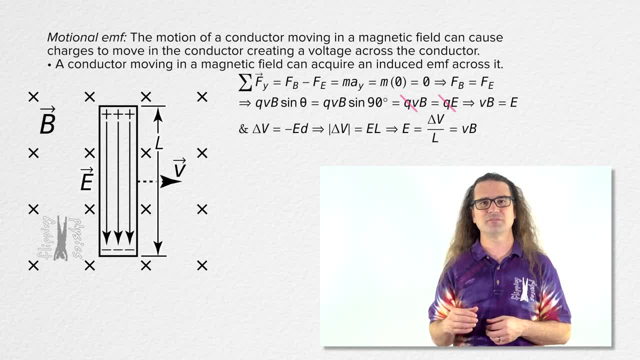 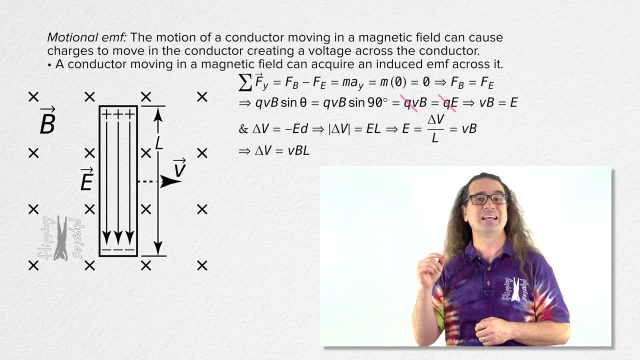 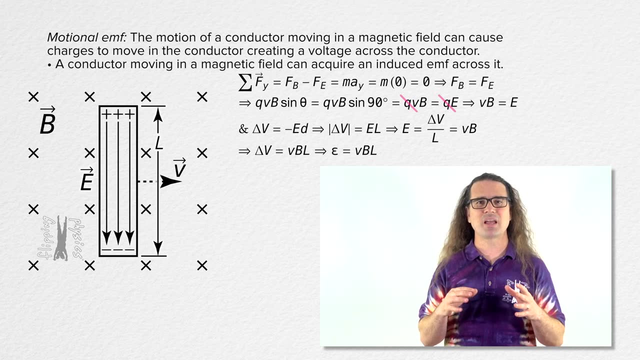 in. We can rearrange that to solve. to get that The induced voltage across the length of the conductor equals the velocity of the conductor times the magnetic field times the length of the conductor. In other words, the motion of EMF built up between the ends of a conductor moving through a constant magnetic field equals the velocity of 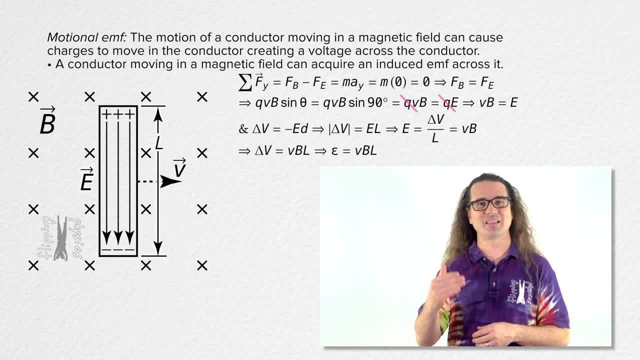 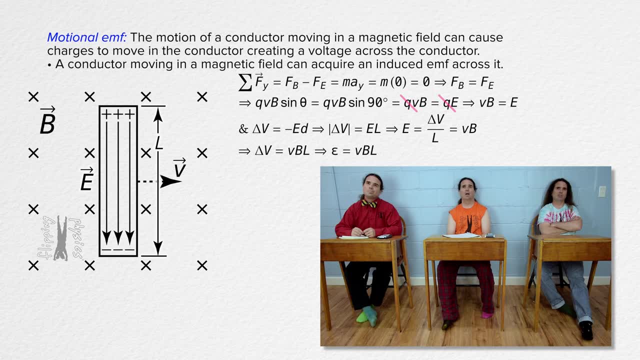 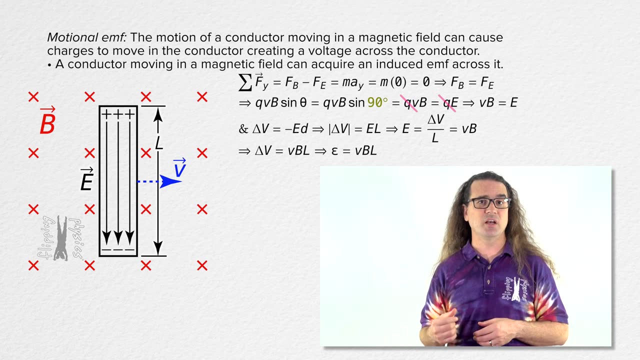 the conductor, times the magnitude of the magnetic field, times the length of the conductor. Again, this is called Motional EMF. But that equation assumes the angle between velocity and magnetic field is 90 degrees right. Valid point Bo. This equation does assume the conductor is moving normal to the plane of the 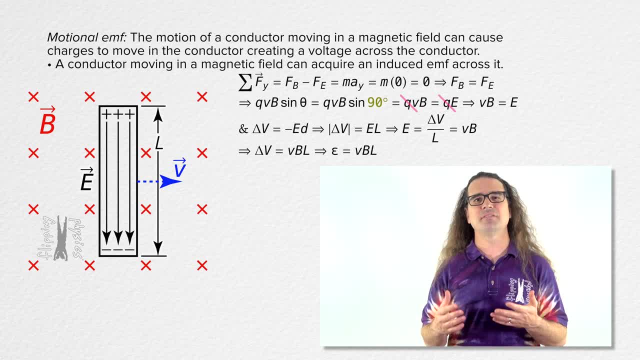 uniform magnetic field. If it is not, you would leave the sine of the angle in the equation. But yes, that is an important thing to realize. Thanks, You're welcome. Now there's actually a completely different way to derive this same Motional EMF equation. 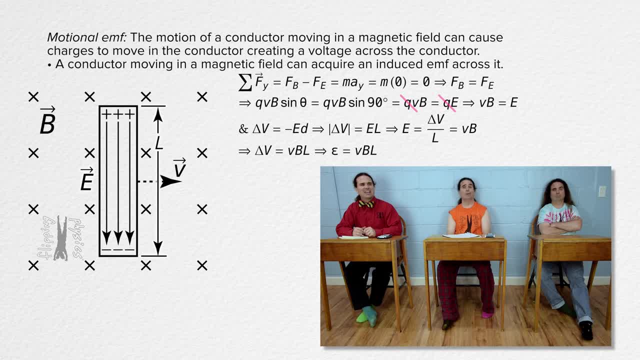 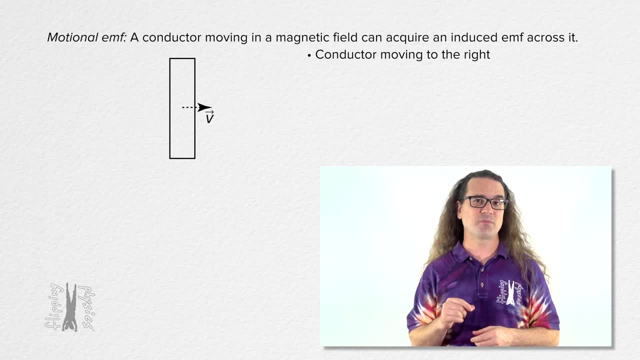 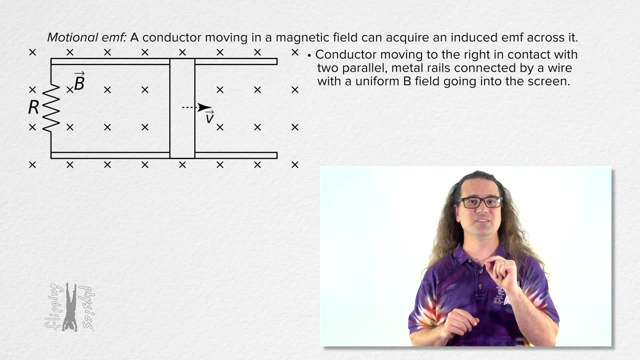 And yes, you do need to know both derivations. You know we love redundancy, We do, Sure, Yeah. This approach starts with a conductor moving to the right while in contact with two parallel metal rails connected by a wire at the left end, with a uniform magnetic field going into the screen. 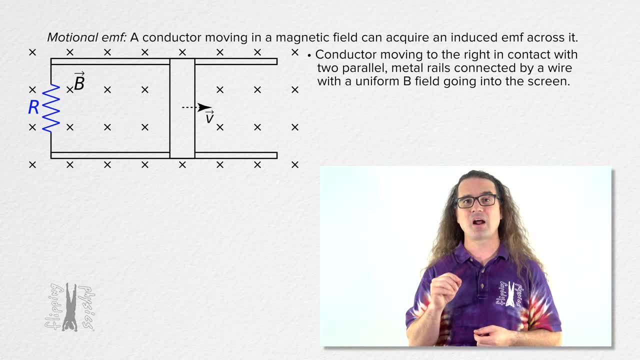 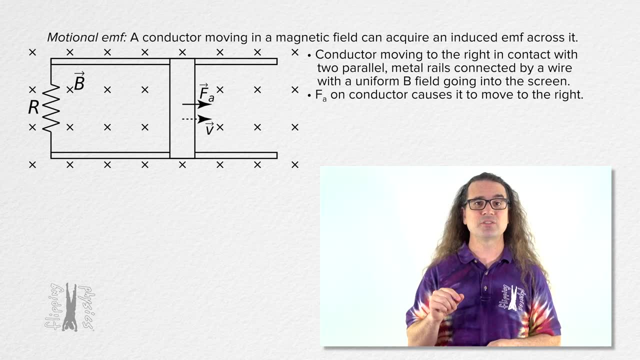 The resistance of the circuit is represented by the resistor shown in the wire on the left. A force is applied to the conductor to cause it to move to the right Notice. a conducting loop is created by the wire on the left, the two parallel conducting rails. 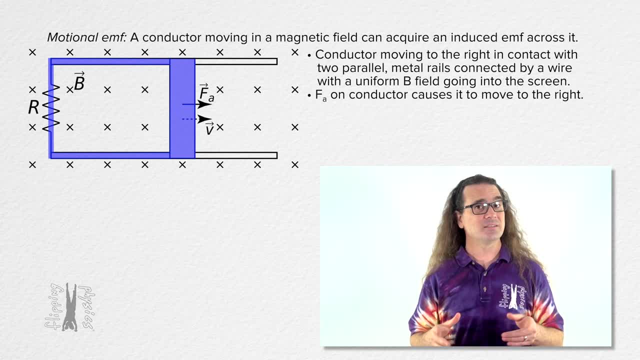 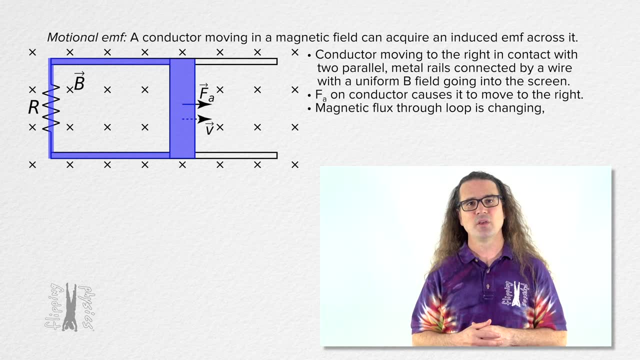 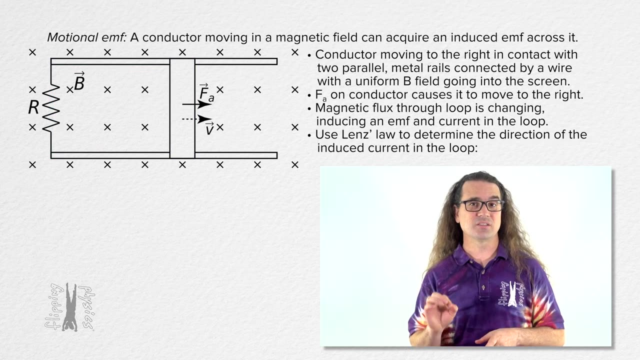 and the conductor which is being pushed to the right And the area of the loop is increasing in size, Which means the magnetic flux through the loop is changing, Which means there is an induced EMF and an induced current in the loop. We can use Lenz's Law to determine the direction of the induced current in the loop. 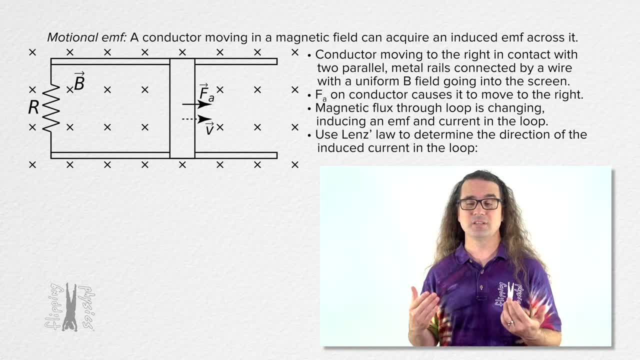 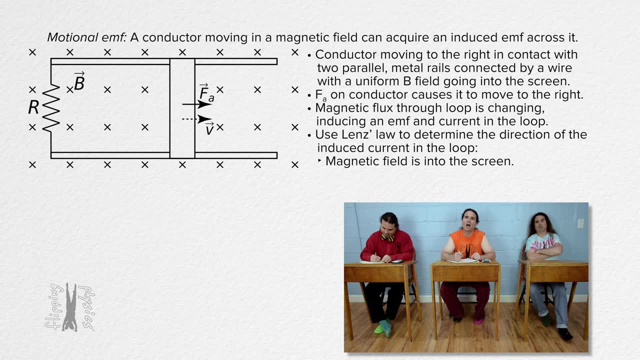 Oh, please determine the direction of the induced current in the loop …. Sure, The magnetic field is into the screen Because the conductor is moving to the right. the area of the conducting loop is increasing in size, So the number of magnetic field lines passing through the loop is increasing, which. 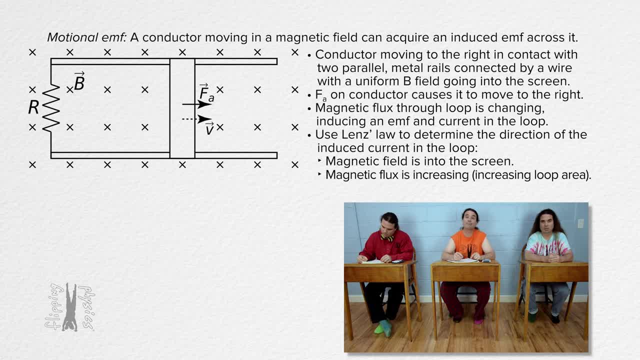 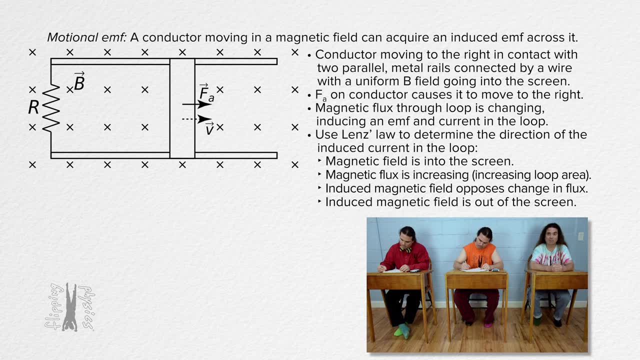 means the magnetic flux is increasing. Yeah, Okay. According to Lenz's law, the induced magnetic field opposes the change in flux. therefore, the induced magnetic field inside the conducting loop is out of the screen. Using the alternate right-hand rule, our fingers curl in the direction of the induced magnetic. 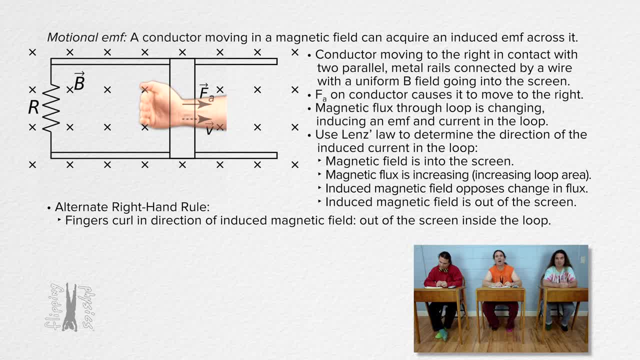 field which is again out of the screen, inside the conducting loop. Our thumb points in the counterclockwise direction from this perspective, which is the direction of the induced current in the loop. Yep, there is an induced current in the loop which is: 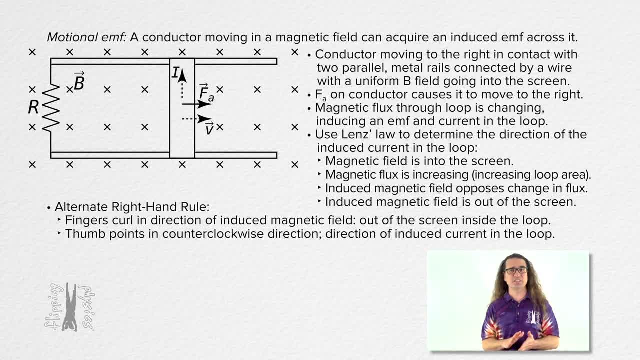 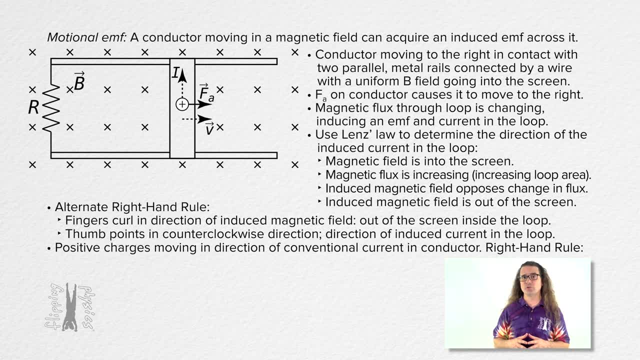 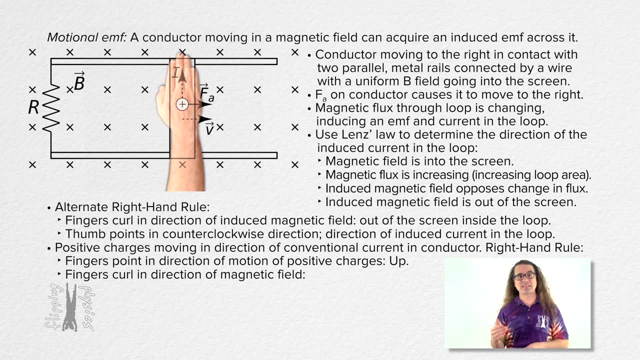 up through the moving conductor. Thanks, Bo Notice. this means that because positive charges are moving in the direction of conventional current in the conductor, we can use the right-hand rule to show that the fingers point in the direction of the motion of the positive charges, which is up. Fingers curl in the direction of the magnetic field. 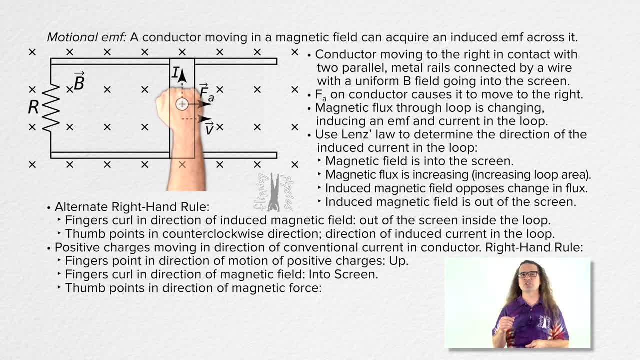 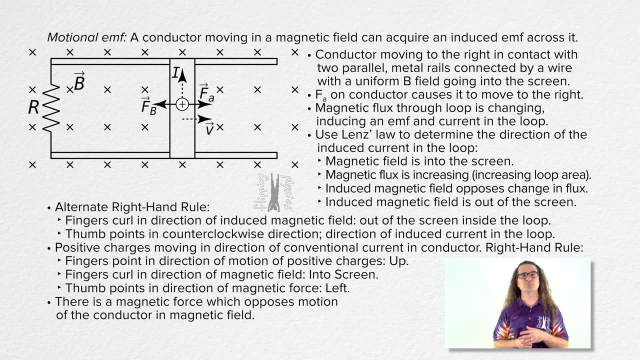 which is into the screen And our thumb points in the direction of the magnetic force on the moving positive charges, which is to the left. In other words, there is a magnetic force which opposes the motion of the conductor in the magnetic field. Realize you get the same result for negative charges moving opposite the direction. 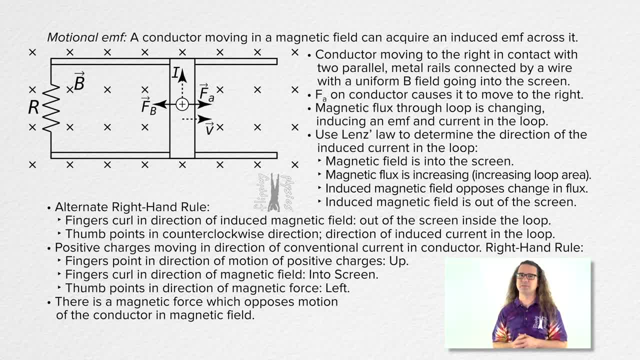 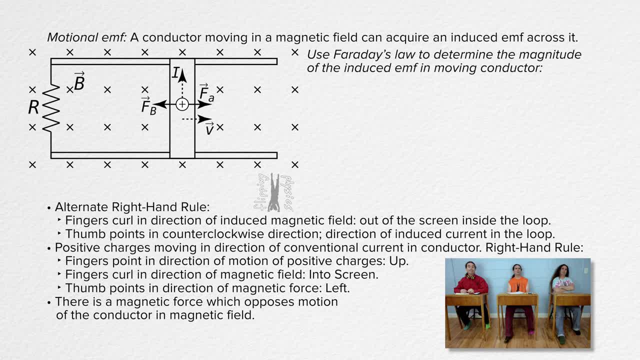 of conventional current in the conductor. Now, Bobby, please use Faraday's law to determine the magnitude of the induced EMF in the moving conductor. Okay, Faraday's law states that the induced EMF in multiple conductive loops equals the negative of. 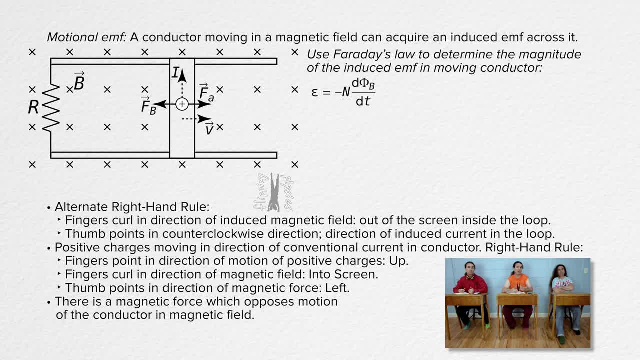 the number of loops. times the derivative of the magnetic flux through a single loop. with respect to time, Magnetic flux equals: the magnetic field times the area of the loops. times the cosine of the angle between the magnetic field and the area of the loops. The number of loops. 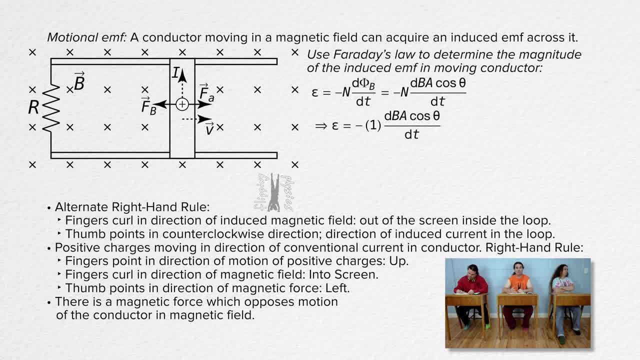 in this case is: 1. The magnetic field does not change over time, so that can be taken out of the derivative. The angle is also constant over time and can be taken out of the derivative. Actually, the magnetic field is into the screen For the direction of the area of the loop. 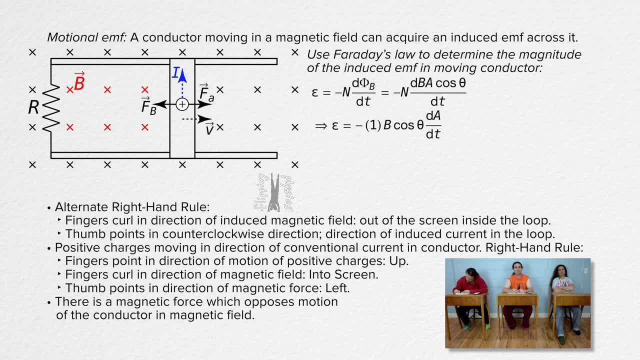 well, the conventional current is counterclockwise from this perspective. so curl the fingers of our right hand counterclockwise and our thumb points out of the screen. so the direction of the area is out of the screen. Okay so because the magnetic 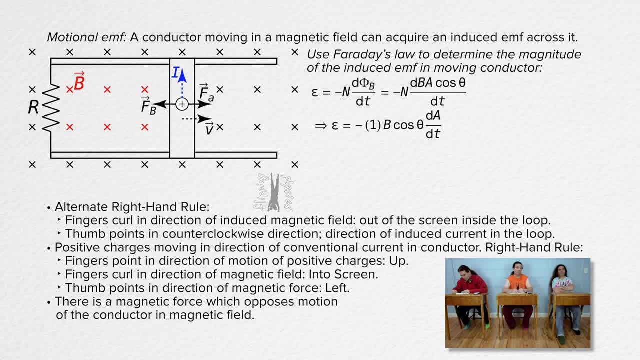 field is into the screen and the loop area vector is out of the screen. the angle is 180.. But what do I do with the area variable? I do not know what the derivative of area with respect to time is. Let's identify the variable: distance the moving conductor is from the wire. 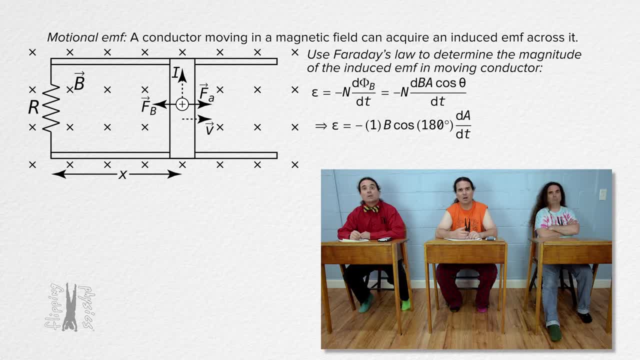 on the left as a variable distance, x. In other words, as the conductor moves to the right, the value of x increases. Sure that makes sense. The area of the loop, then, is capital L times x, and is constant over time, which means we can take L out from the derivative and the derivative of 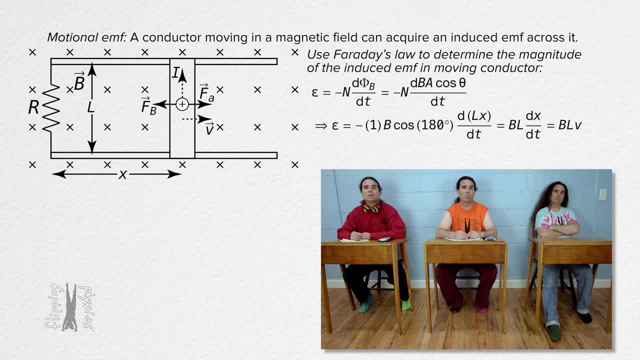 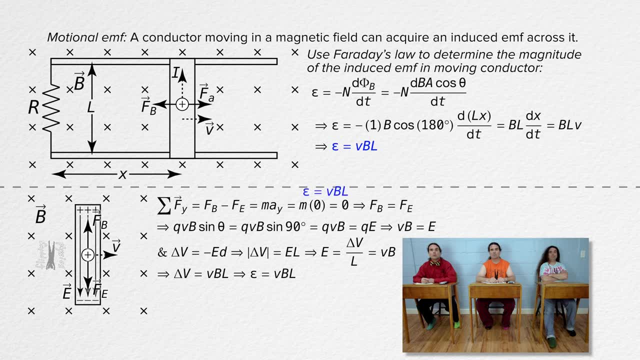 x position with respect to time is velocity. We just derived the same equation for emotional EMF as we did before. Emotional EMF equals velocity times, magnetic field times the length of the conductor, And again this equation assumes the angle between the velocity of the conductor and. 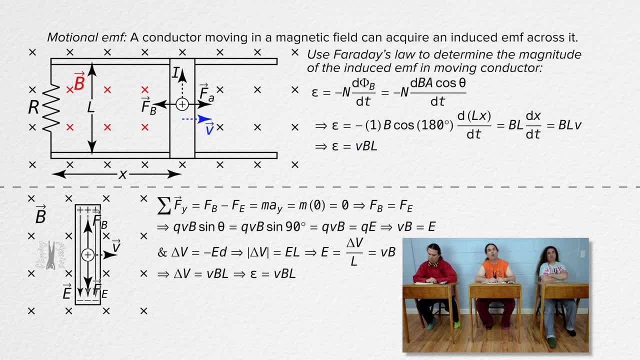 the magnetic field is 90 degrees. If it is not, you can leave the angle in the equation. But the way we did it before had the sine of theta in it. This way has the cosine of the angle instead, This way of deriving the emotional EMF equation. 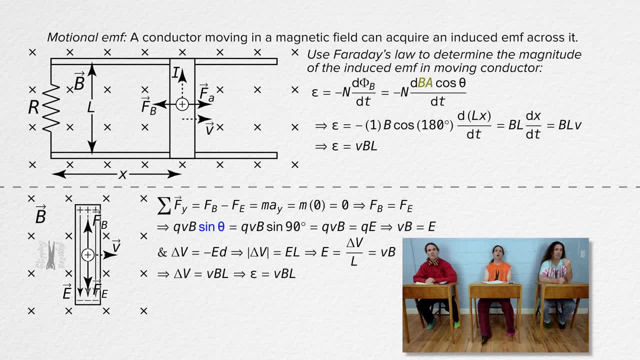 defines theta as the angle between the loop area vector and the magnetic field, The way we did it before defined theta as the angle between the direction of the velocity of the conductor and the magnetic field. The loop area vector and the velocity of the moving vector are at a right angle to one another, which is why one of these equations uses cosine. 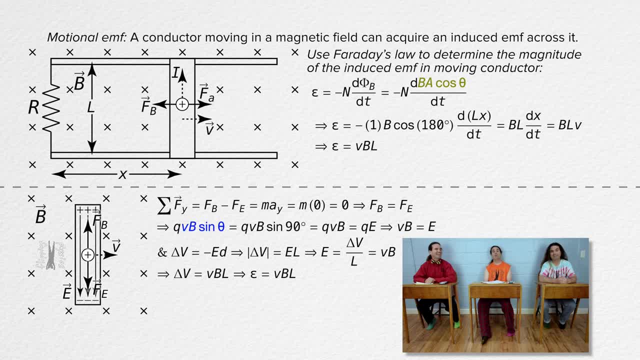 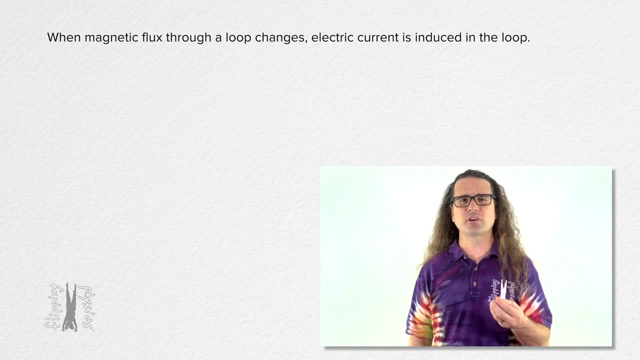 and the other uses sine. Okay, Thank you everybody, Well done. Up to this point, we have discussed how, when magnetic flux through a loop changes, electric current is induced in the loop. What we haven't yet discussed is how the magnetic field 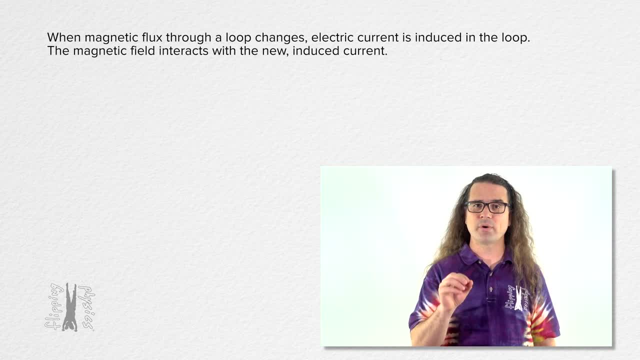 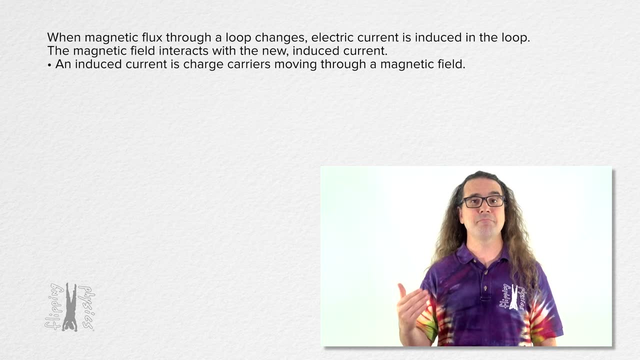 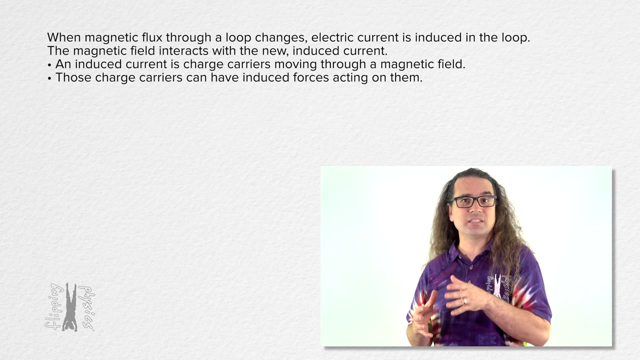 then interacts with the new induced current. That is what we are about to learn about. Realize an electric current is a bunch of charge carriers which are moving in a magnetic field, That induced current. those moving charges can also now have induced forces acting on them. as a result, 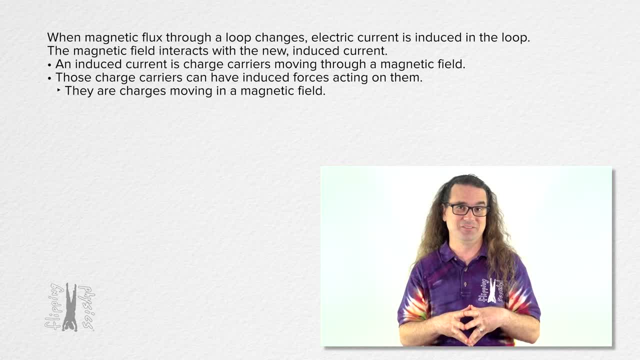 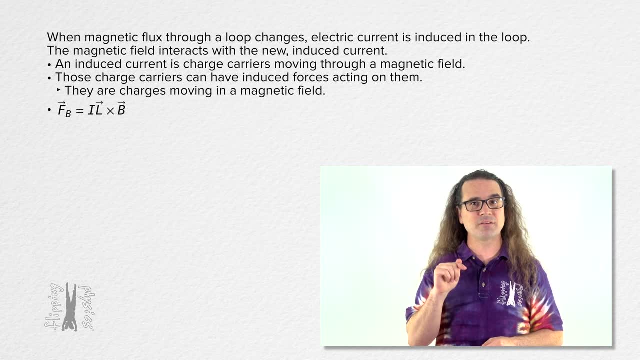 of the fact that they are charges moving in a magnetic field. The magnetic force on a current carrying wire equals the cross product of current times, the length vector of the wire and the magnetic field. This equation is for when the current is constant. the wire is straight. 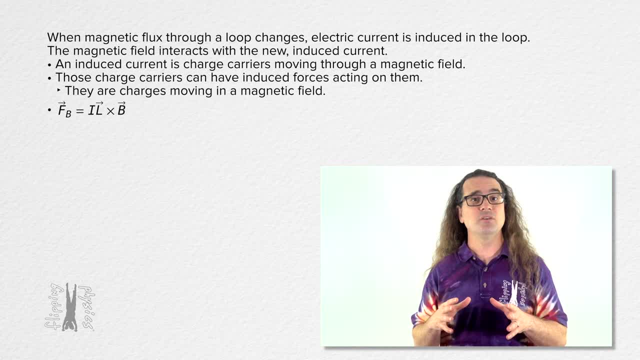 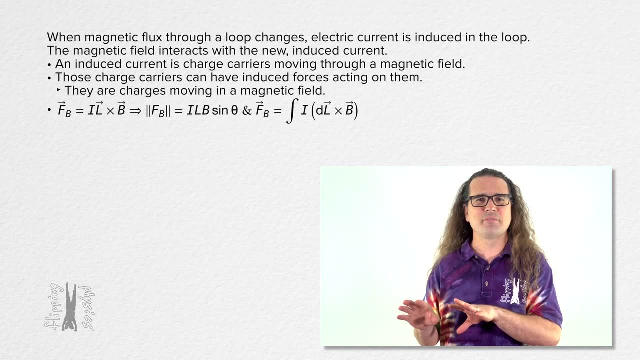 and the magnetic field is uniform and constant And we also have the magnitude of the magnetic force equation. We're not going to concern ourselves with the integral form of the magnetic force equation right now because we are only going to look at straight wires and uniform, constant magnetic. 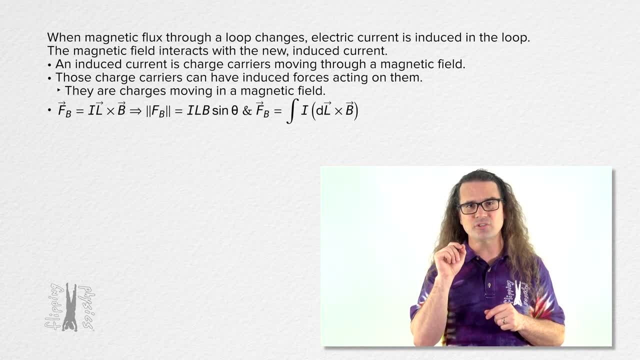 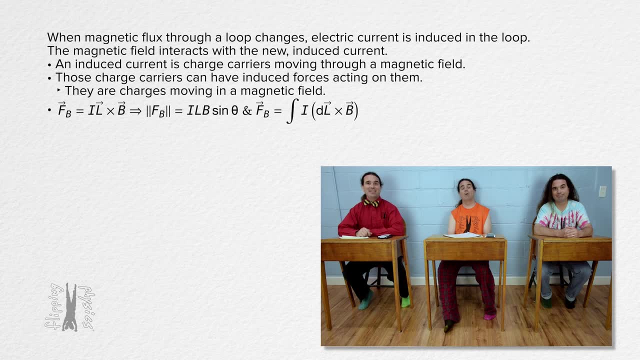 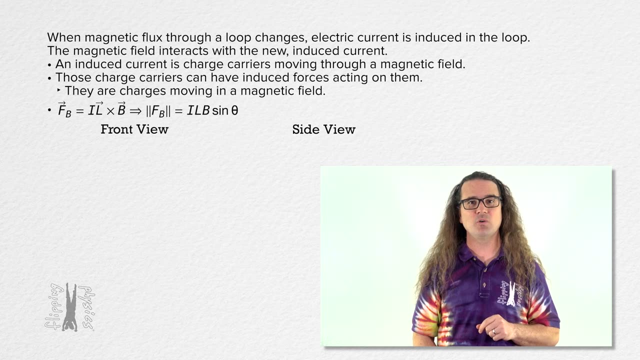 fields, Because what I'm really interested in making sure you understand right now concerns the directions of the induced magnetic forces on induced currents. Can we do an example? Yes, Billy, Let's do an example. Goody, I love examples. In our example we have a front view and a side view of the magnetic force equation. 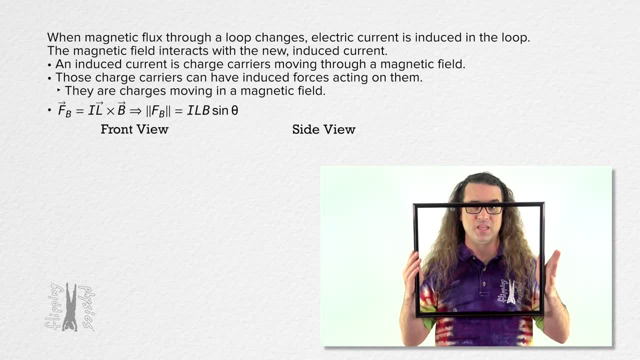 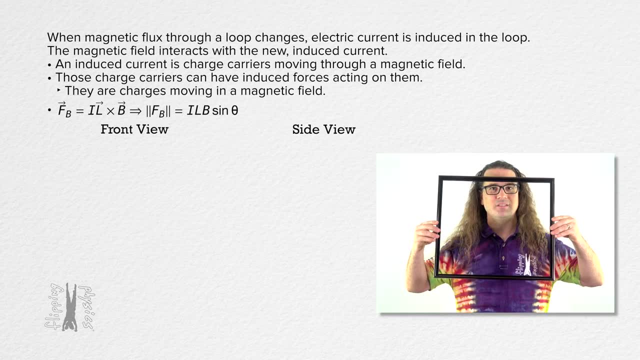 Let's take a look at a conducting loop in the shape of a rectangle. Basically, we have a wire rectangle in the shape of a picture frame And that conducting wire loop is oriented like this: In the front view you can see there is a uniform magnetic field which is coming toward you. 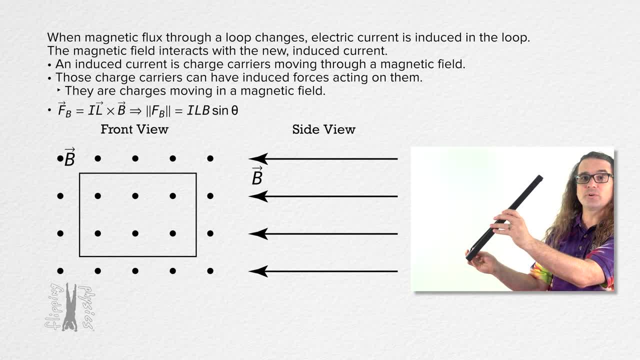 In the side view, the uniform magnetic field is going to your left and the rectangular conducting wire loop is oriented like this. Again, the front view looks like this, with the uniform magnetic field coming toward you- toward you- and in the side view, the uniform magnetic field is going to your left. 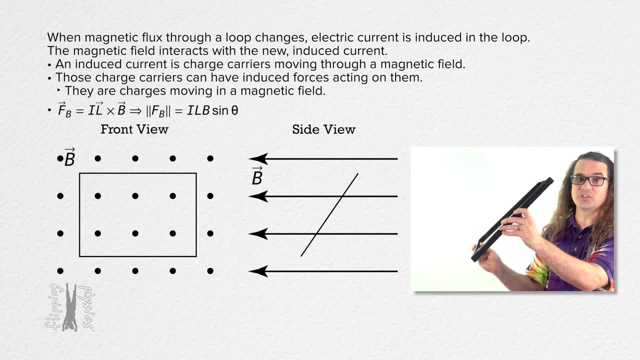 Now I am about to talk about a lot of directions, and every direction I will be referencing will reference the front view. Again, every direction I'm about to mention is in the perspective of the front view. I think we get it, Mr P? Yeah, right now, you think that? 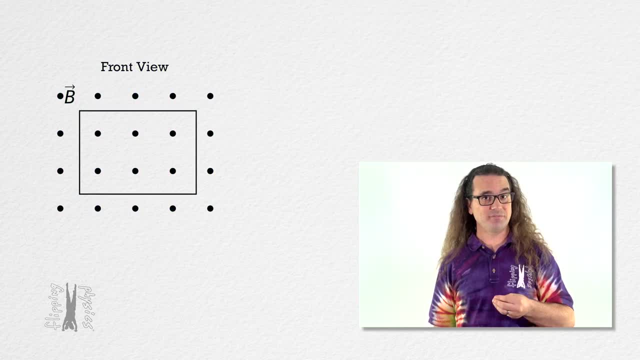 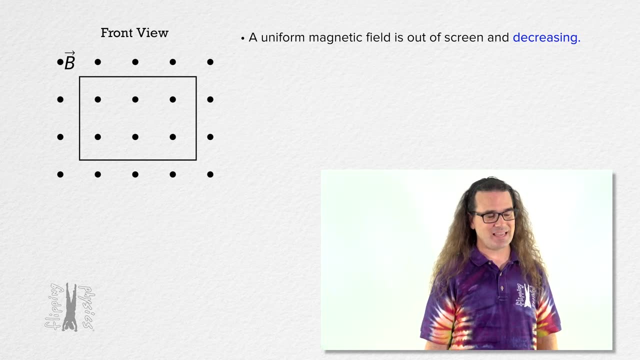 Yep, Okay. The uniform magnetic field, which is out of the screen, is decreasing in magnitude. Billy, what does that mean for the direction of the induced current in the rectangular loop? A uniform magnetic field is out of the screen and decreasing. 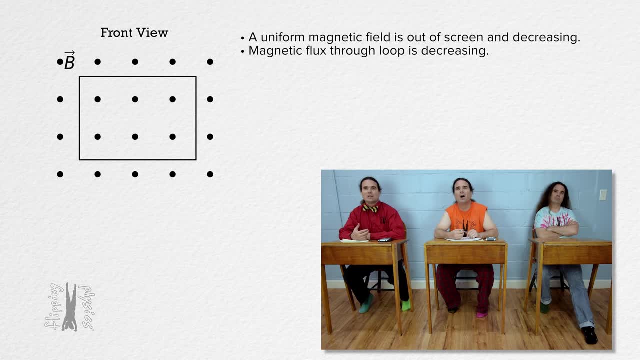 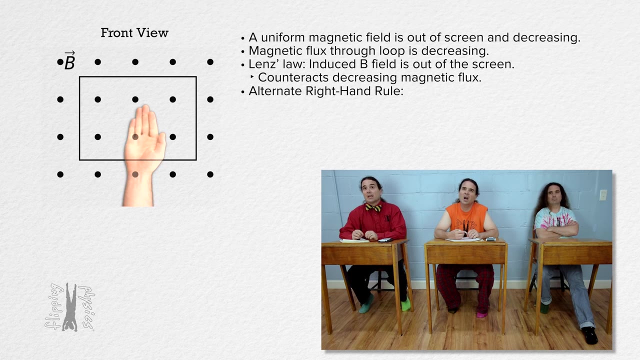 That means the magnetic flux through the loop is decreasing. Lenz's Law tells us the induced magnetic field opposes that change in magnetic flux. therefore, the induced magnetic field inside the loop is out of the screen. Using the alternate right-hand rule, I'm already limbered up. 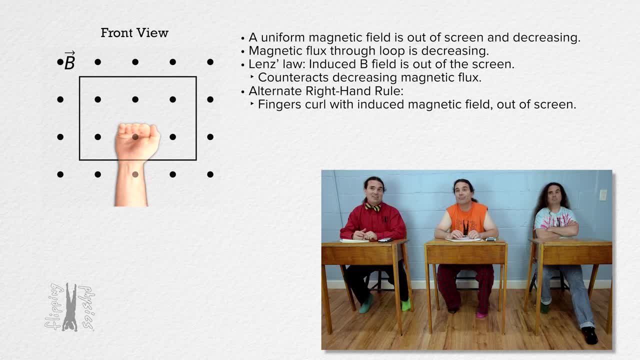 Fingers curl. The induced magnetic field inside the loop which is out of the screen thumbpoints counterclockwise with the induced current in the loop. The induced current in the loop is counterclockwise from the front view perspective. Thanks, Billy. 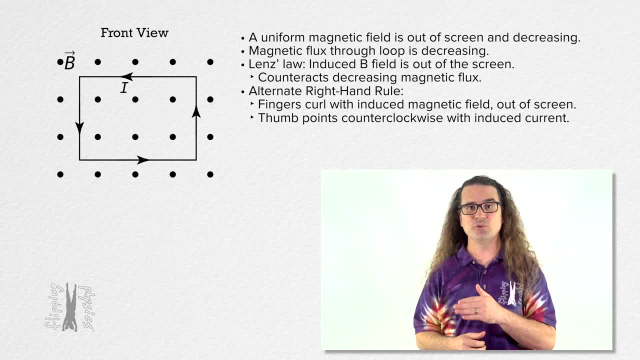 Now to talk about the induced magnetic forces on the induced current in all four sides of this rectangular conducting loop. let's give each side a number. Side 1 is on the top. Side 2 is on the right. Side 3 is on the bottom. 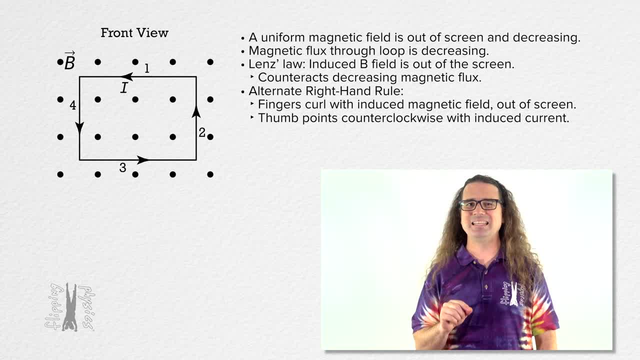 Side 4 is on the left. Please notice I have not given each of the currents in all four sides of the loop subscripts because they all have the same magnitude current. It is the induced current caused by the decreasing magnetic flux through the loop. 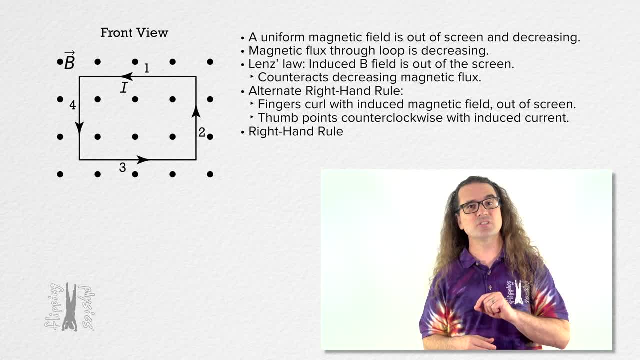 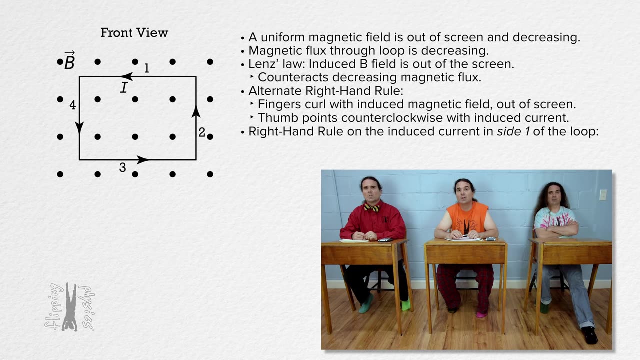 Bo, please use the right-hand rule to determine the directions of the induced magnetic forces caused by the induced currents in this uniform magnetic field. And again, every direction referred to right now is still in the front view. Sure Side 1 has current going to the left. 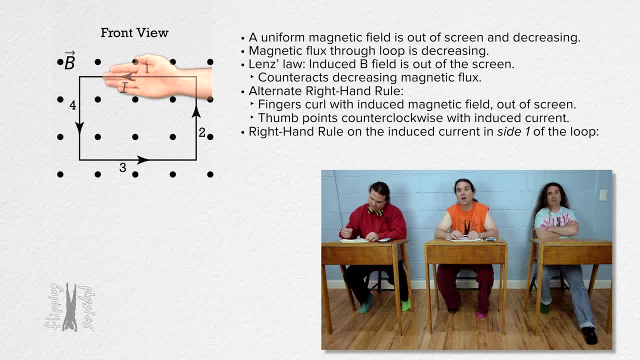 So point the fingers of my right hand to the left. I too am already limbered up And clearly not too cool. Duh, Side 1, pointing figures to the left with the current Fingers curl out of the screen with the magnetic field. 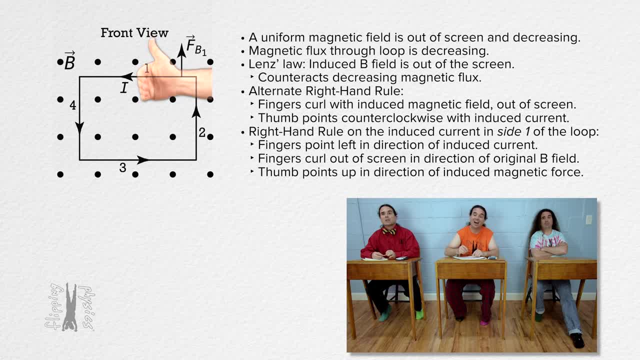 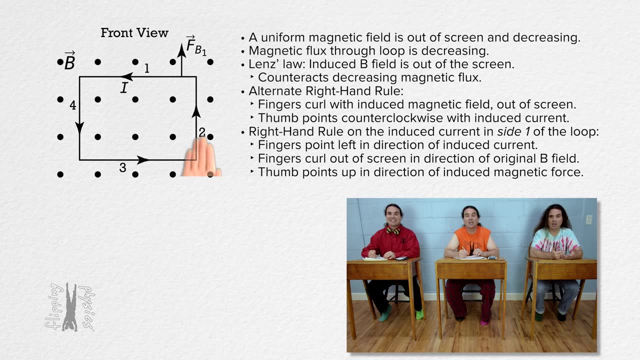 Thumb points up in the direction of the induced magnetic force on side 1 caused by the induced current passing through side 1, which is in A magnetic field. Thanks, The other 3 sides. Okay For side 2.. Fingers point up with the current. 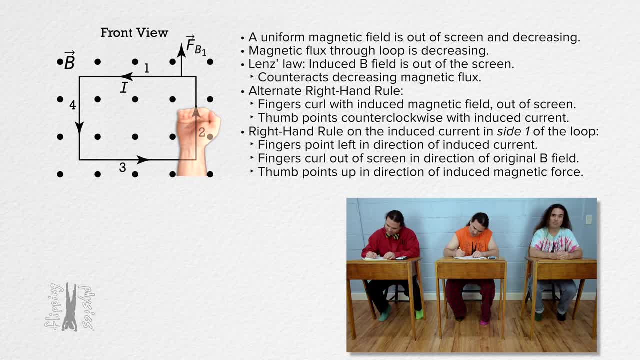 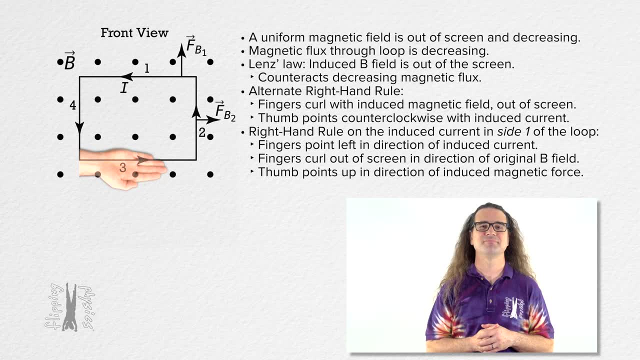 Curl fingers out of the screen with the magnetic field. Thumb points to the right in the direction of the induced magnetic force on side 2.. For side 3.. Fingers with current to the right Curl out of the screen with magnetic field. 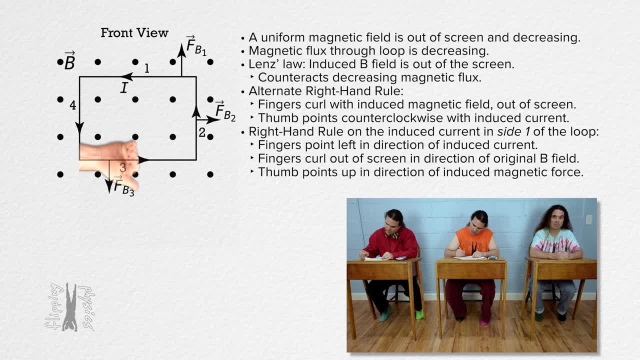 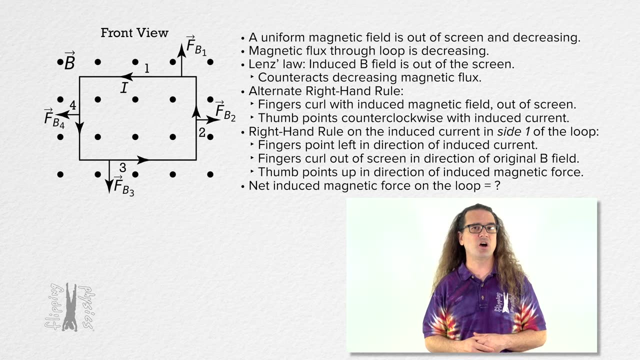 Thumb points down: C on side 3.. For side 4, fingers point down with current curl out of the screen. thumb points left with magnetic force on side 4.. Thank you, Bo. Now, Billy, please determine the net force caused by. 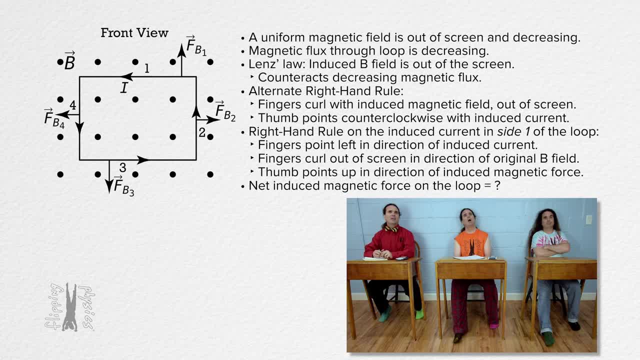 all the induced magnetic forces on the rectangular loop. How do I do that? I mean we don't have any numbers Interesting. So, Billy, are you telling me you have a numbers dependency? I do not have a numbers dependency, It's just…. 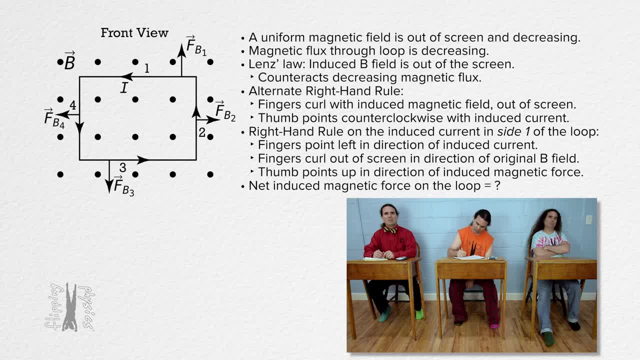 Start by looking at just sides 1 and 3.. Oh, okay, The induced magnetic force is on sides 1 and 3.. Okay, I think I see. The magnitude of the induced magnetic force equals the current times the length of the wire, times the magnitude of 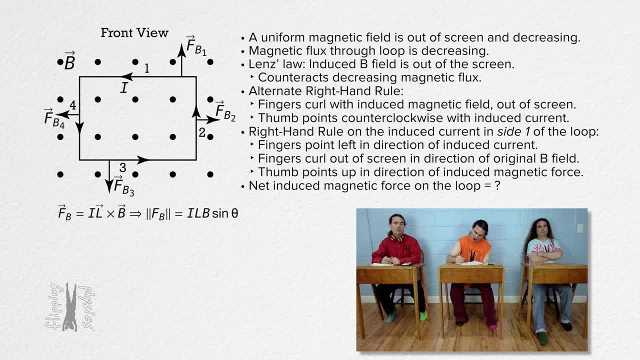 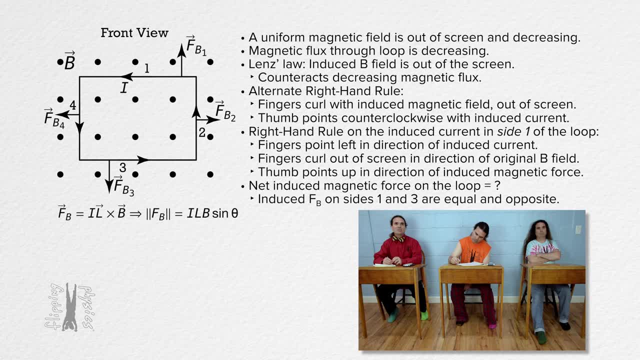 the magnetic field Times, the sine of the angle between the two, For sides 1 and 3,. all of those values are the same. The currents are the same, the lengths of the wires are the same, the magnitudes of the magnetic 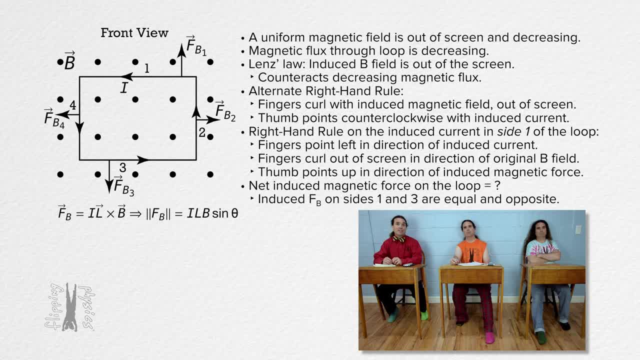 fields are the same and the angles are the same And the directions of the magnetic forces are opposite to one another. That means the net induced magnetic force on sides 1 and 3 of the rectangle equals zero, And the same is true for sides 2 and 4.. The current has the same magnitude. 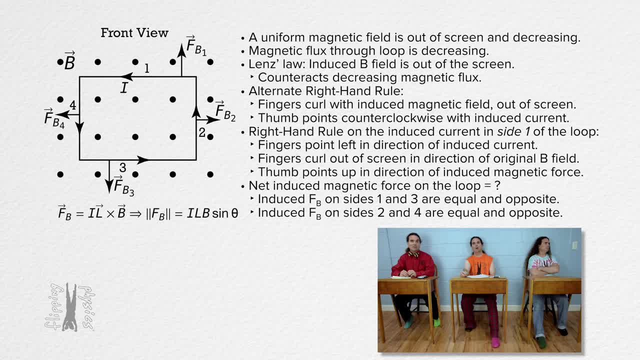 the lengths of the wires are the same, the magnetic field has the same magnitude at the locations of both sides, 2 and 4, and the sine of the angle for sides 2 and 4 gives the same value. So the net induced magnetic force for sides 2 and 4 is also zero, And that means that the 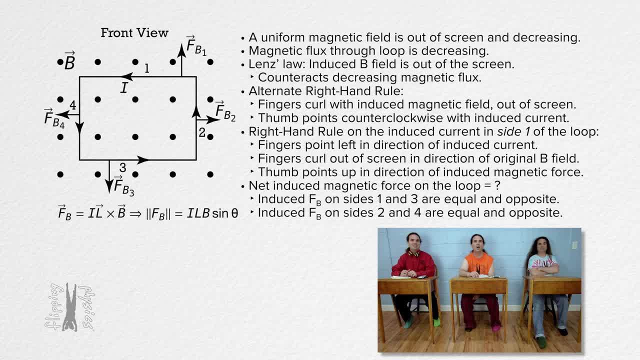 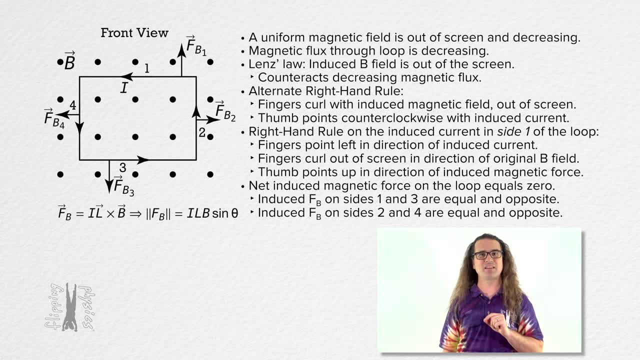 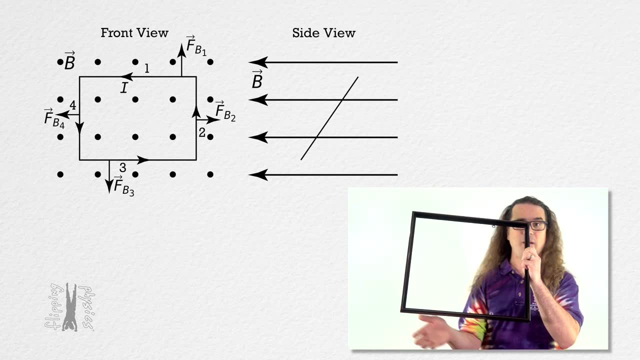 net induced magnetic force on the entire rectangular loop equals zero. No numbers dating Nice, Very nice. The net induced magnetic force on this current carrying loop in a uniform magnetic field is zero. Now let's switch from the front view to the side view. Again, this represents the 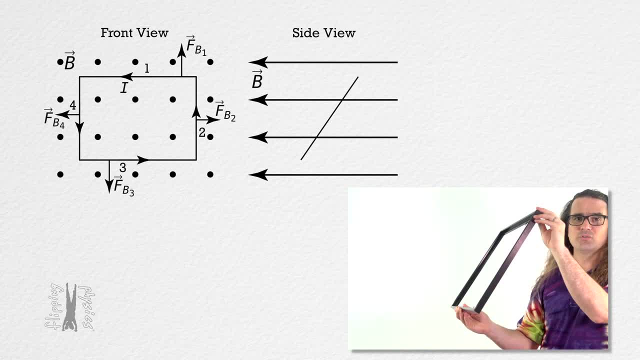 rectangular loop in the front view. This is the rectangular loop in the front view. This is the rectangular loop in the front view And this represents the rectangular loop in the side view. Bobby, please walk through the directions of the current and induced magnetic forces on. 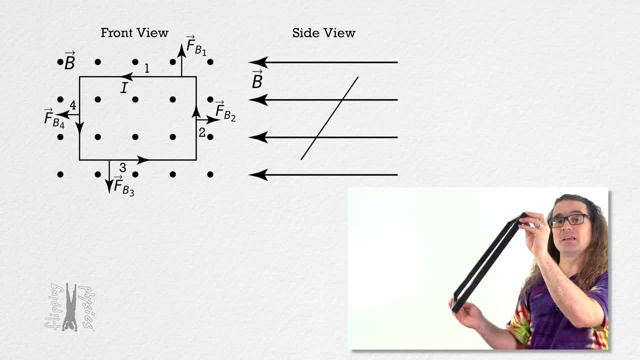 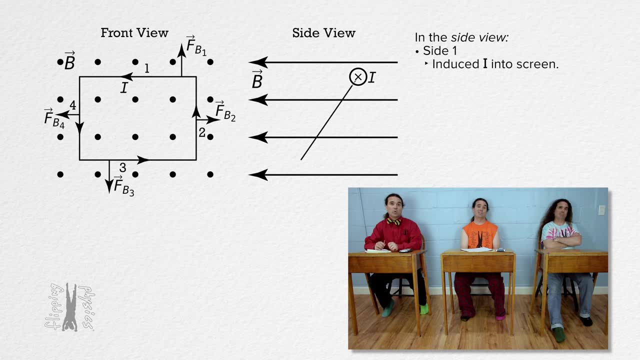 all four sides of the rectangular loop only now in the side view. Yeah, I can do that In the side view. the current through side 1 is into the screen And the induced magnetic force on side 1 is up. The current through side 2 is up and to the right And the 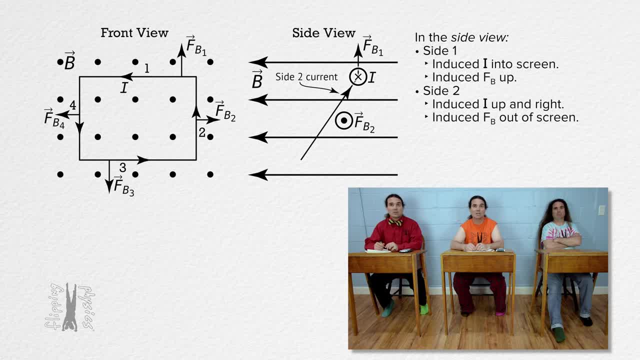 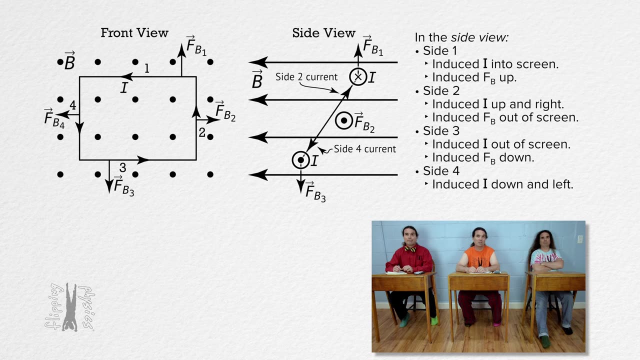 magnetic force on side 2 is out of the screen, The current through side 3 is out of the screen And the induced magnetic force on side 3 is down. The current through side 4 is down and to the left And the induced magnetic force on side 4 is into the screen. 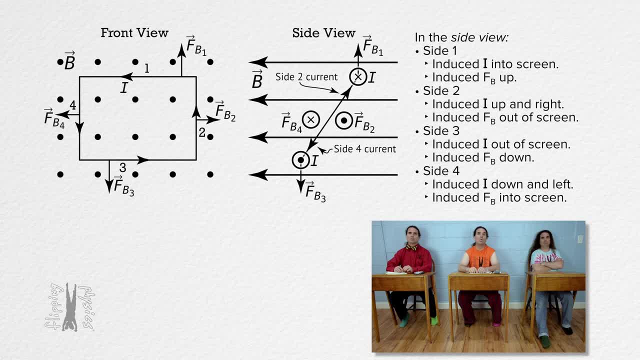 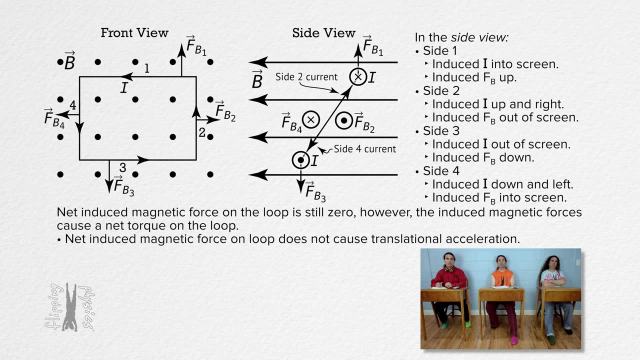 Okay, I think I see what you are getting at. While the net force caused by the induced magnetic forces on the rectangular loop equals zero, there is actually a non-zero net torque on the rectangular loop. The net induced magnetic force on the loop does not cause a translational acceleration of the loop. However, the induced 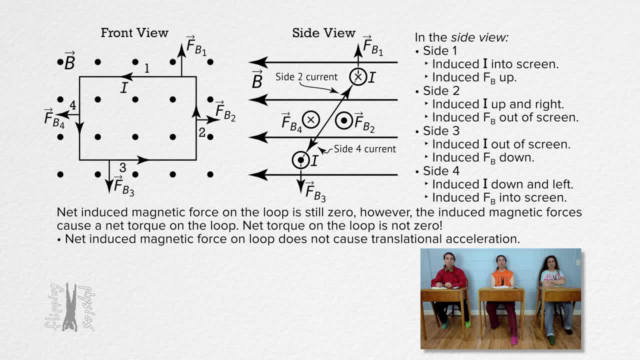 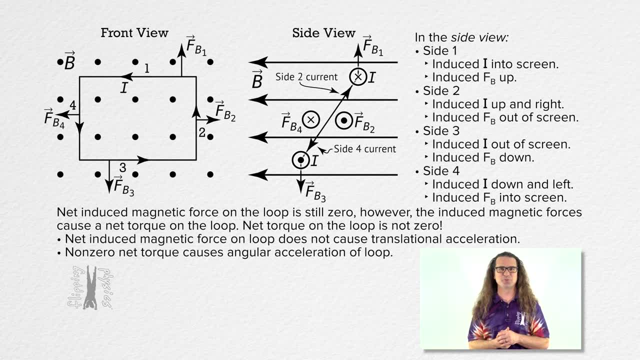 magnetic force causes a net torque on the loop, which can cause an angular acceleration of the loop. That's pretty cool. Yes, that is pretty cool. In this example, assuming the loop is not attached to anything, the net torque on the loop would cause an angular 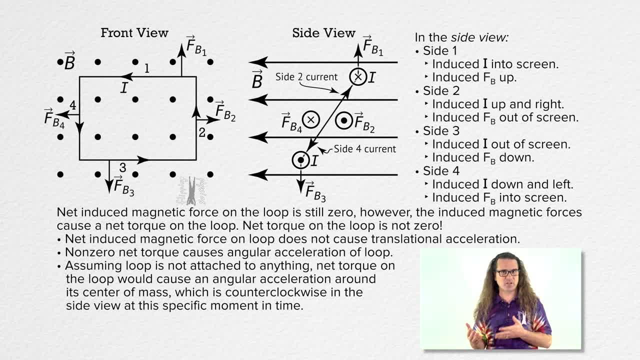 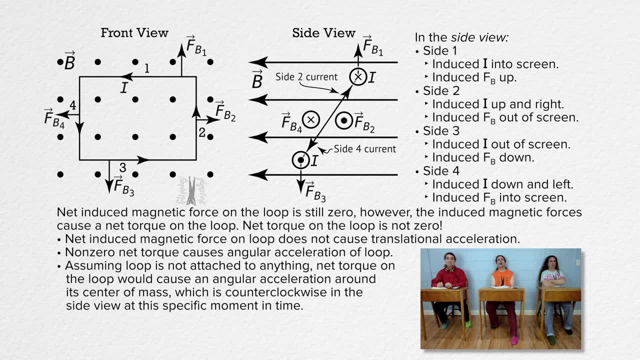 acceleration around its axis. The net torque on the loop would cause an angular acceleration around its center of mass, which is counterclockwise in the side view perspective. At this specific moment in time, The loop would have a force of gravity acting downward, causing a downward translational. 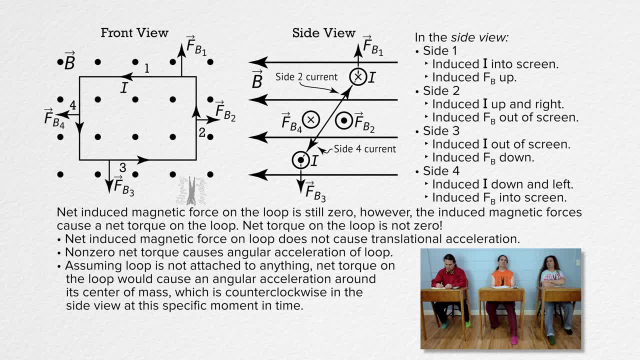 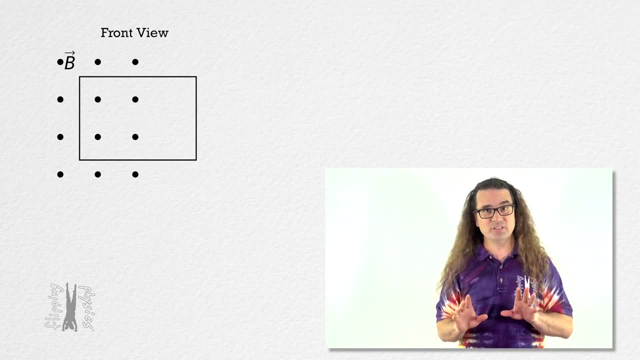 acceleration right? I think this is all theoretical right now, and he's ignoring the force of gravity acting on the loop. He is Sure that's fine. Now let's change the example by making it so: the magnetic field ends abruptly part way through the loop, As you can see. 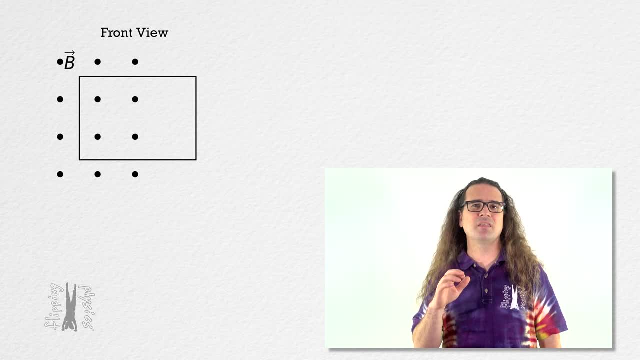 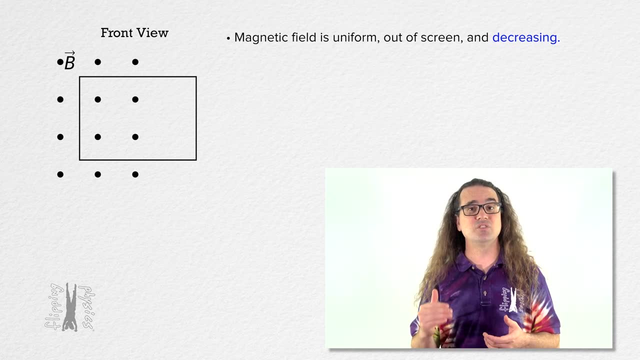 in the front view the magnetic field only exists inside roughly the left half of the rectangular loop. Again, the magnetic field is uniform, directed out of the screen and decreasing in magnitude. Lenz's law gives us the same counterclockwise direction in the front view for 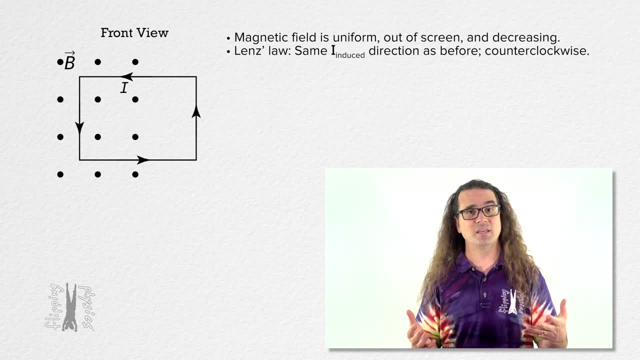 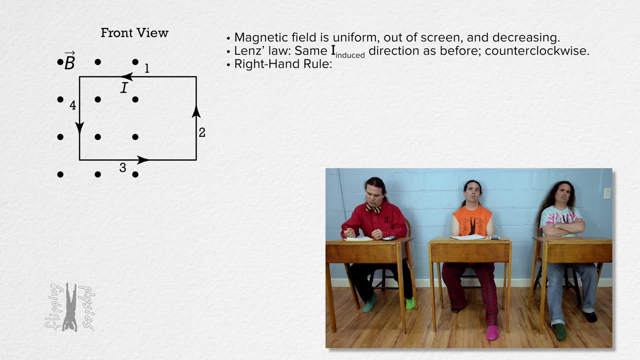 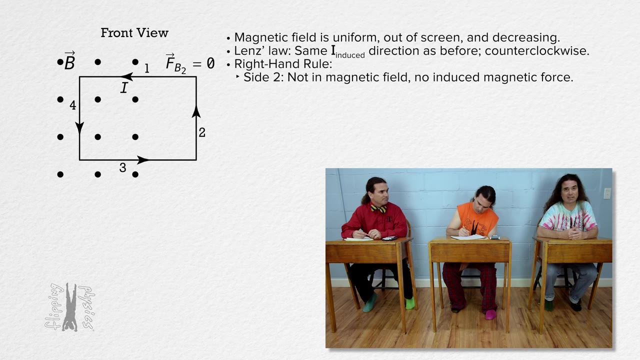 the induced current in the loop Bo. please again determine the directions of the magnetic forces on the four sides of the conducting rectangle. Sure Well, let's actually start with side 2, because… Side 2 is not in a magnetic field, so there is no induced magnetic force on side 2.. 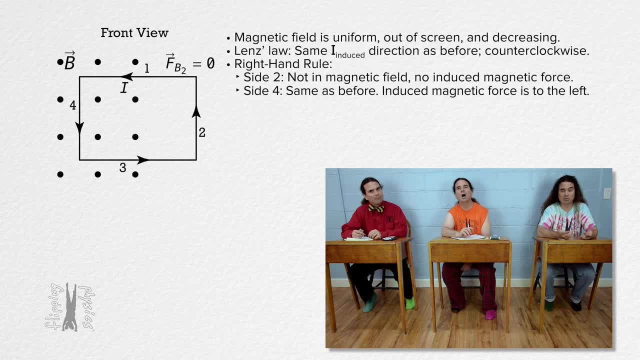 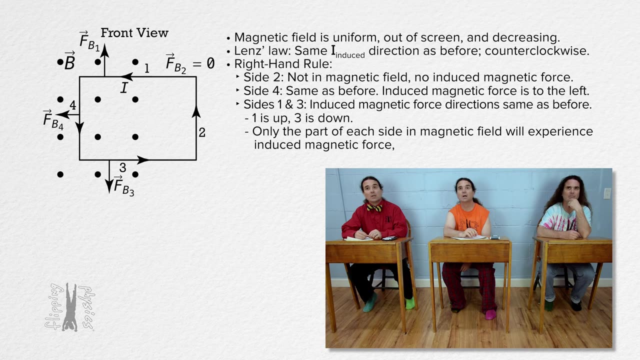 Everything is the same for side 4.. The induced magnetic force on side 4 is to the left. For sides 1 and 3, the directions of the magnetic forces are the same as before. Side 1 is up, side 3 is down. However, the length of the wires inside the magnetic 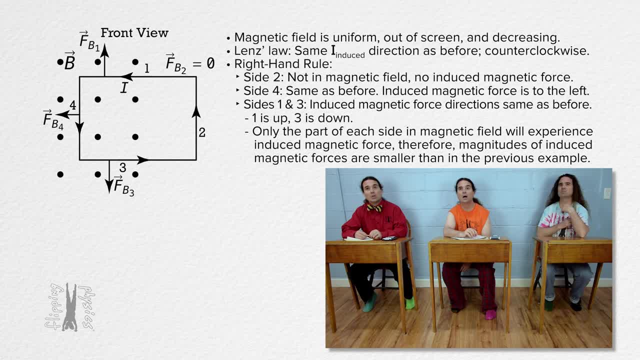 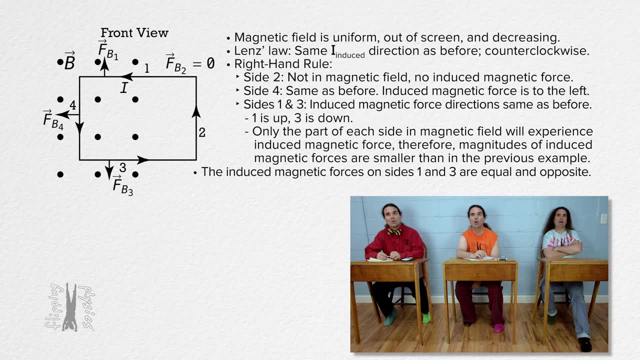 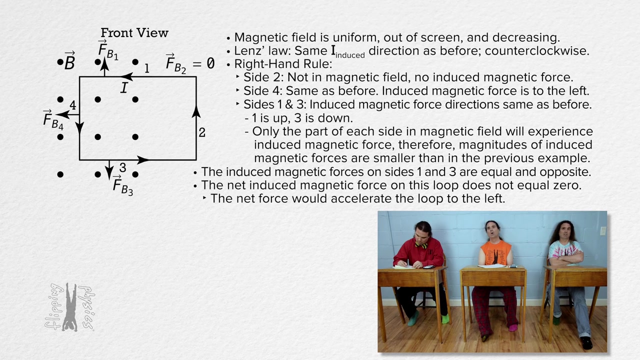 field has decreased. Therefore the magnitudes of the induced magnetic forces are also decreased. But those two forces are still of equal magnitude and still cancel one another out. So the net induced magnetic force on this entire loop is no longer zero. The net induced magnetic force on this loop is to the left, so this loop would accelerate to the left. Correct, Bo thanks, And we can now give the general statements that…. The net induced magnetic force on a current carrying loop which is entirely in a uniform external magnetic field always equals zero. However, those induced magnetic forces can cause a net torque on the loop. And the net induced magnetic force on a current carrying loop. 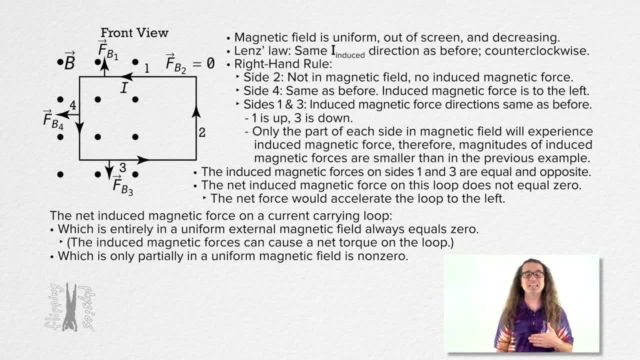 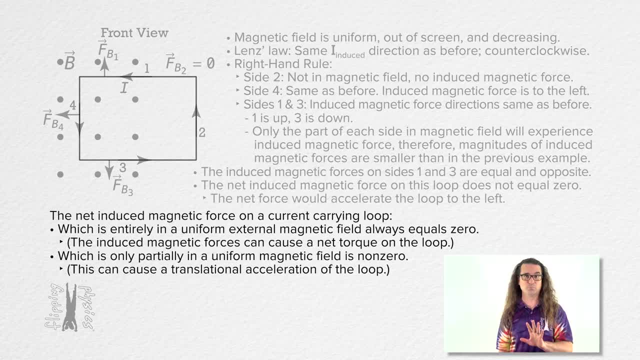 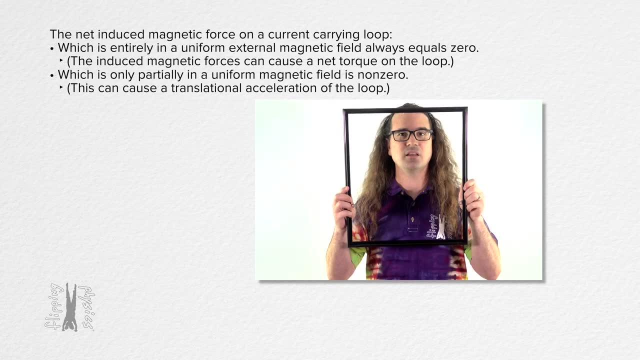 which is only partially in a uniform magnetic field, is non-zero. And this non-zero net induced magnetic force can cause a translational acceleration of the loop. Alright, another example: Again, we have a rectangular conducting loop, A rectangular wire loop, in a uniform magnetic field, oriented like this. 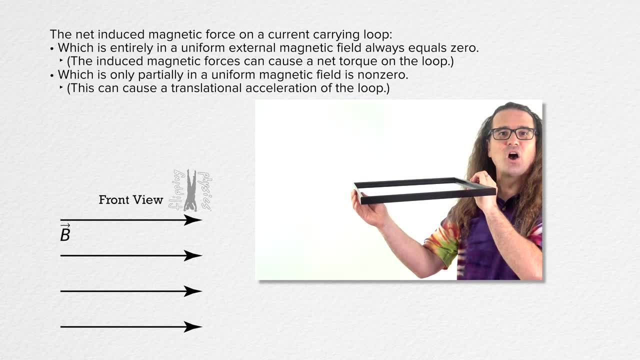 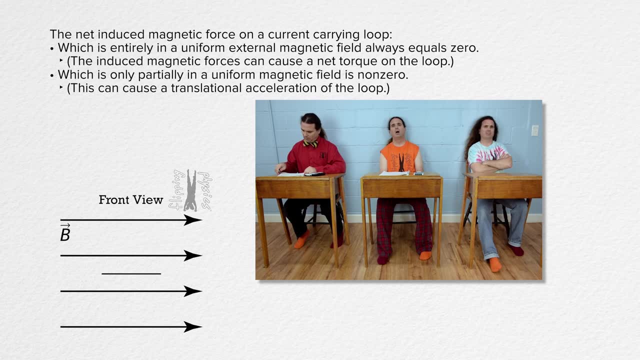 Recognize that in the front view, all you are going to see of the rectangular conducting loop is a straight line representing one side of the loop. Hold up, I don't get it. Did you just say the magnetic field is oriented like this? I don't get it. What is like this? 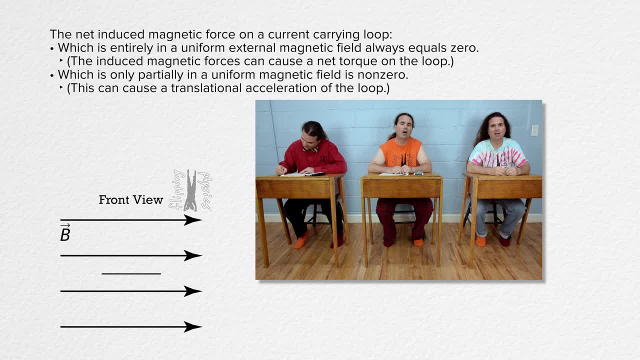 Oh, I'm sorry, Bo. I can see how that was confusing. What I meant to say was…. What I meant to say is that in the front view, the magnetic field is to your right and the loop is oriented like this: Okay, I guess that makes sense. 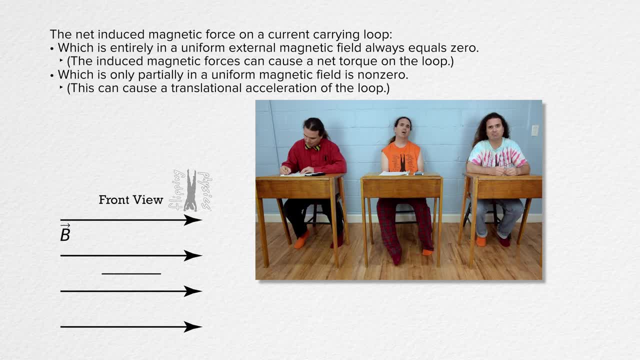 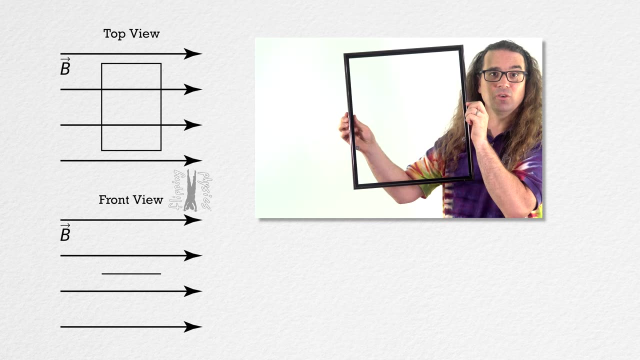 The magnetic field is to the right. Okay, Yes, And again, just to be absolutely clear, in the front view, all you are going to see of the rectangular conducting loop is a straight line representing one side of the loop. When you look at the loop from the top view, you get the top view and you can. 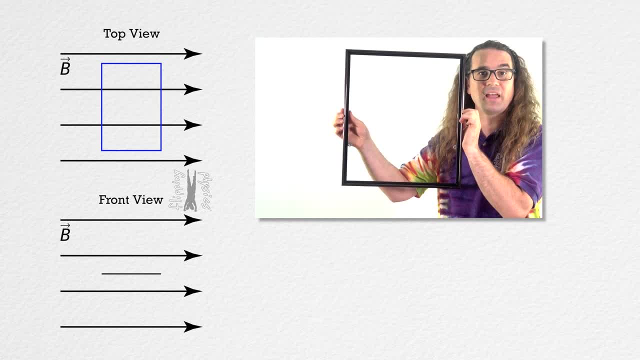 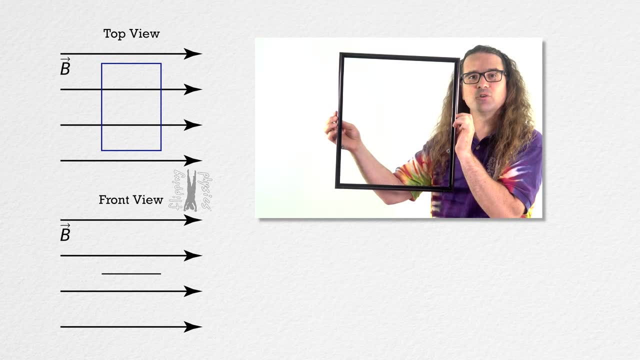 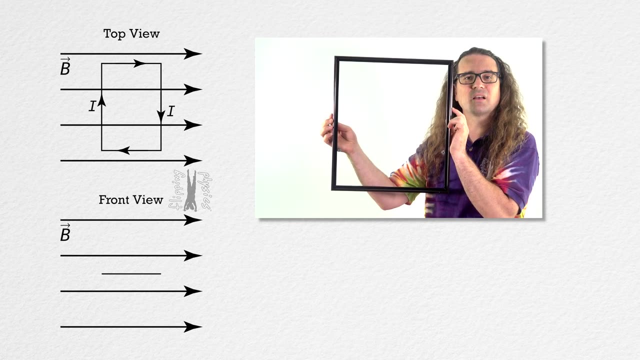 now see the full rectangular conducting loop which I am again using a picture frame to represent. In this example we are going to place an EMF across the loop to cause current capital. I in the loop In the top view you can see the current we are placing on the loop is clockwise. 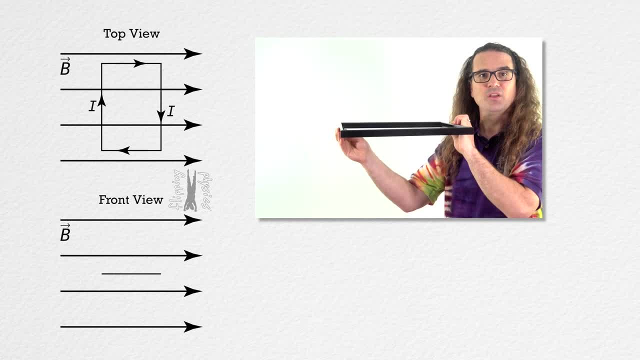 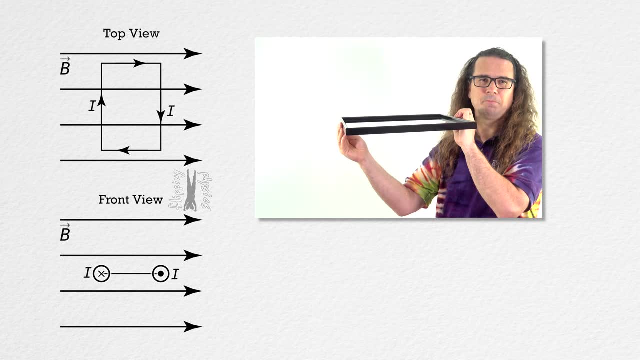 This means, when, looking at the front view, the current is coming out of the screen on the right side of the loop and the current is going into the screen on the left side of the loop, Because conventional current represents the motion of positive charges in the wire. 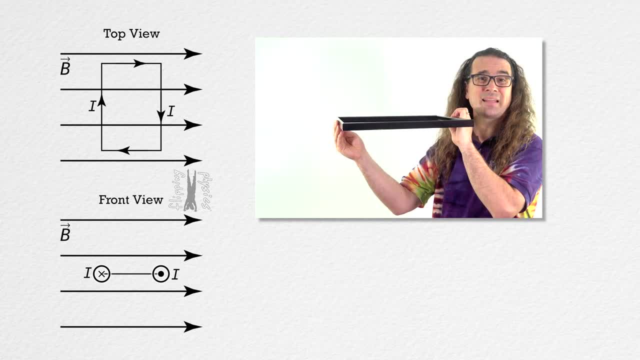 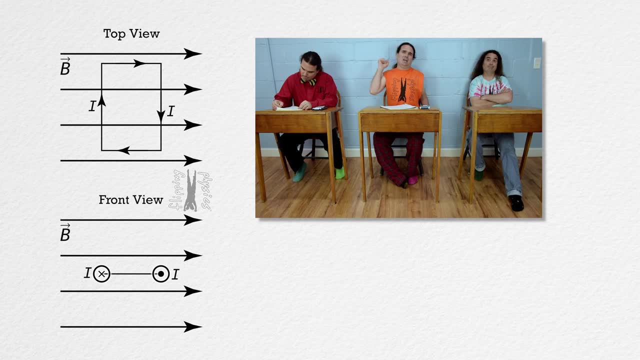 we can use the right-hand rule to determine the directions of the induced magnetic forces on in the front. view the left and right sides of the loop. Bobby, please do that For the current coming out of the screen on the right side of the rectangular loop in the front. 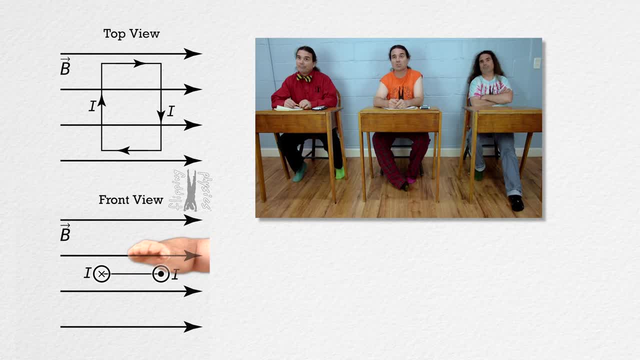 view. fingers point out of the screen in the direction of the current. fingers curl to the right in the direction of the magnetic field. Thumb points up in the direction of the induced magnetic force on the right side of the loop For the current going into the screen on the left side of the rectangular loop. 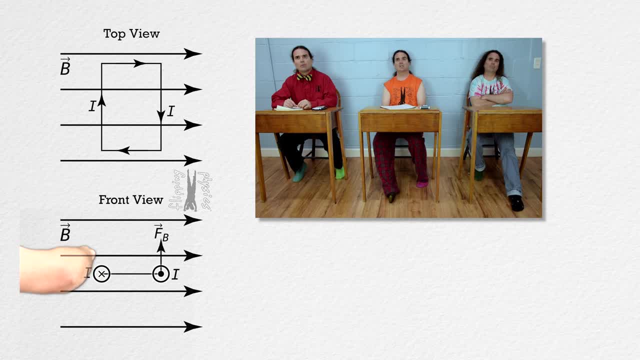 still in the front view. fingers point into the screen in the direction of the current, fingers curl to the right in the direction of the magnetic field and thumb points down in the direction of the induced magnetic force on the left side of the loop. Oh, okay, I get it. There is a net torque acting on the loop. 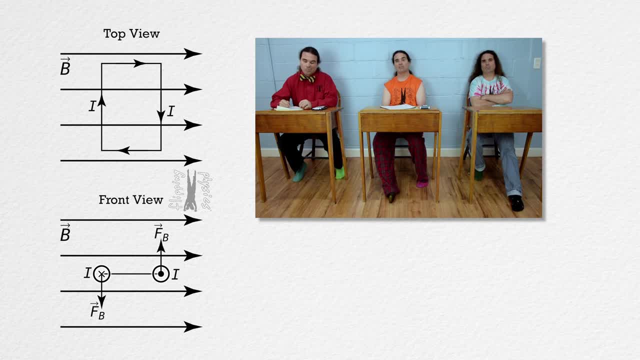 from the current passing through the wires in the uniform magnetic field, Exactly, And let's add an insulated hinge in the middle of the rectangular loop which allows the current carrying loop to rotate around that axis of rotation. You can see, I have added that axis of rotation in the top view and in the front view And I have 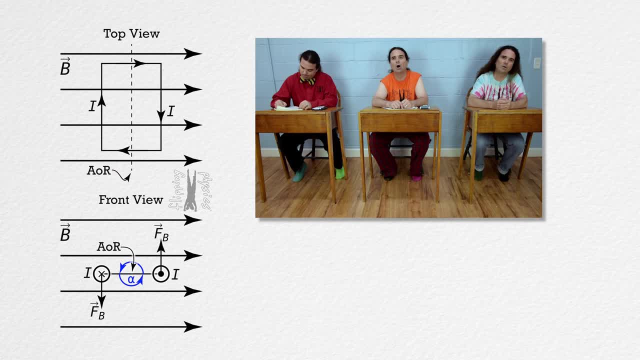 shown that the wire loop will angularly accelerate in the counterclockwise direction. in the front view, In the top view, the induced magnetic force on the wire on the right side is out of the screen and the induced magnetic force on the wire on the left side is into the screen Right, Mr P. 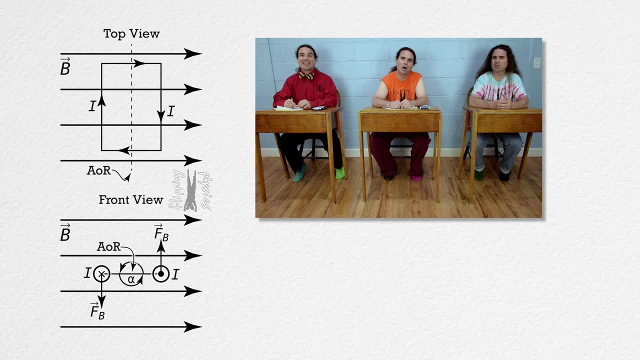 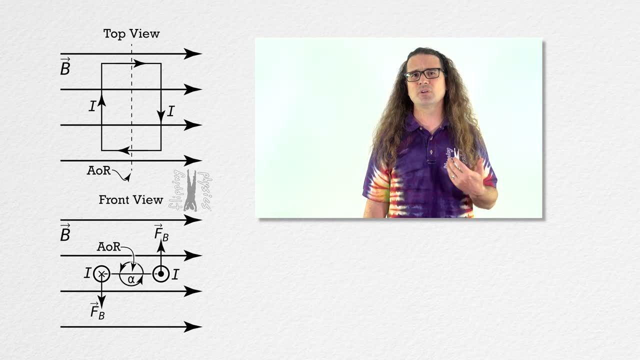 Why are we not adding those to the illustration? Yes, Bo, you are correct. Honestly, there is so much going on here that if I were to include everything in these illustrations, they would be so crowded that they would not help. you see what? 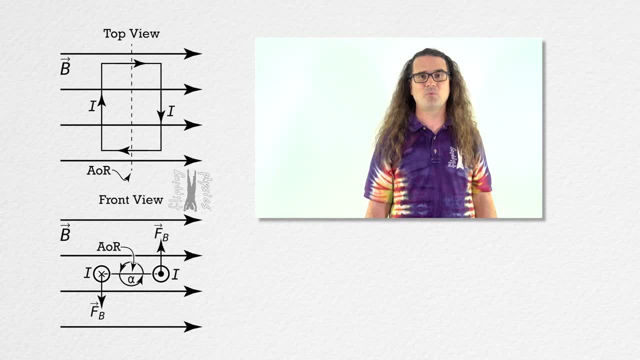 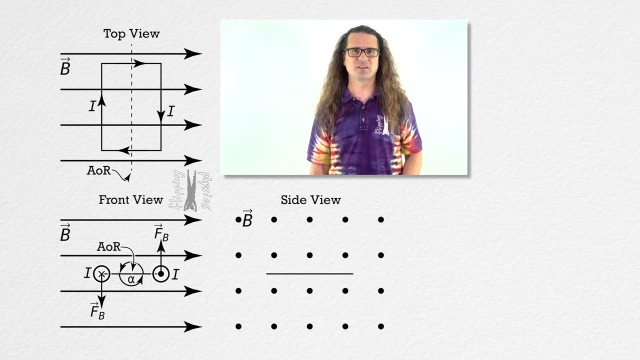 is going on, So I am being selective about what I show you in the illustrations. For example, I need to add a side view so we can understand what happens. Okay, So again, this represents the rectangular conducting wire loop from the top. This: 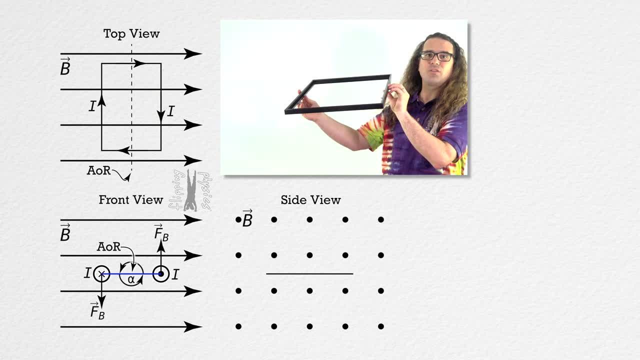 represents the conducting wire loop from the front, And this represents the conducting wire loop from the side. In the side view, all you see is the one side of the wire loop, which looks just like a line, And the axis of rotation around which the wire loop rotates. 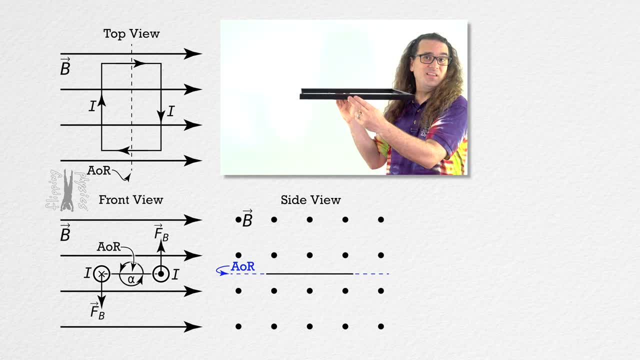 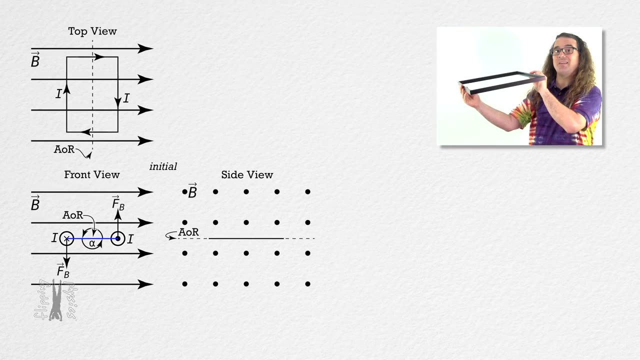 passes through that line, And this is just the initial position of the rectangular conducting wire loop. As we showed, there is a net torque acting on the loop which causes it to angularly accelerate In the front view perspective in the counterclockwise direction. After the loop has 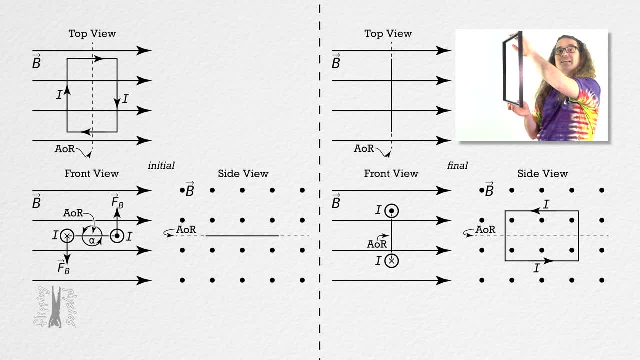 rotated 90 degrees, we arrived at what I am identifying as the final position of the rectangular conducting wire loop. Again, in the front view, the wire loop rotates from the initial position here to the starting position of the rectangular conducting wire loop. So 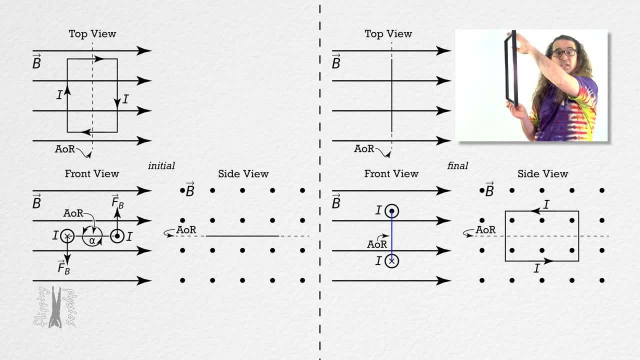 to the final position here. In this final position, in the top view, the loop looks like a line. In the front view, the loop also looks like a line And in the side view you can see the rectangular shape of the loop. At this final point in the front view, you can see the current. in the top. 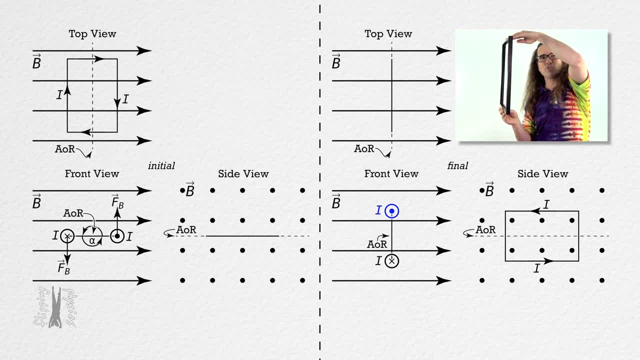 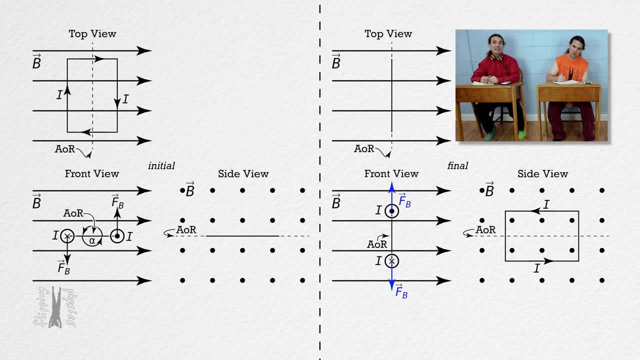 wire is still out of the screen, causing an induced magnetic force which is still upward. The current in the bottom wire in the front view is still into the screen, causing an induced magnetic force which is still downward. That means there is zero net torque caused by the induced magnetic forces on the loop at the 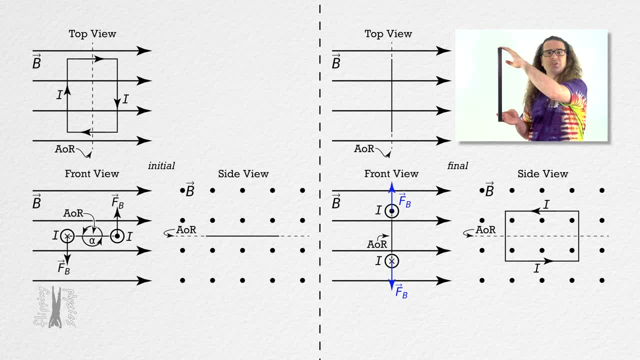 final position, right, Mr P? That is correct, Billy, And notice that the current which is out of the screen in the top wire in the front view is to the left in the top wire in the side view, And the current which is into the screen in the bottom wire in the front view is to the 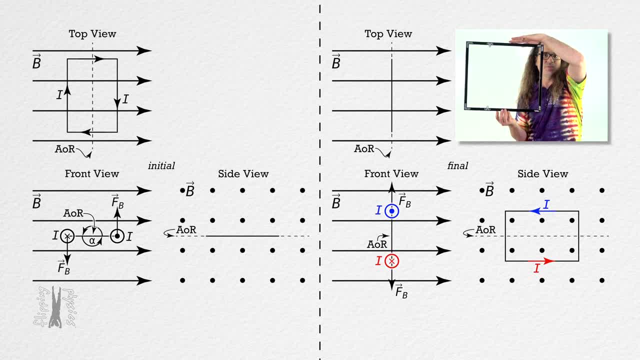 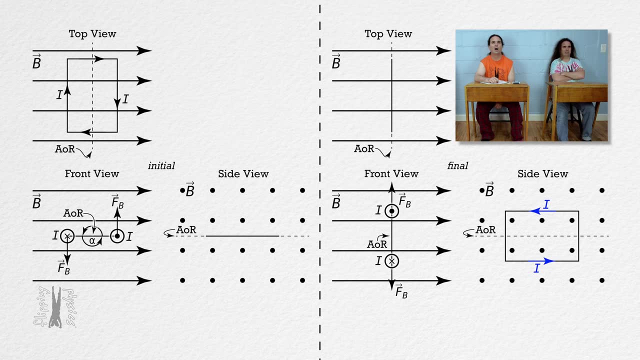 right in the bottom wire in the side view. That means the current in the wire loop in the final position in the side view is counterclockwise. You know this is a lot. You're just talking about current passing through a wire loop in a magnetic field, right, I mean. 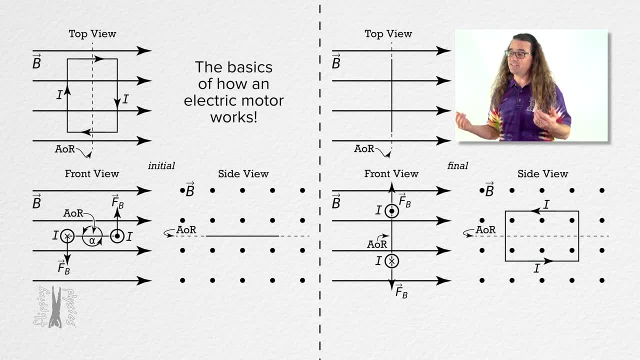 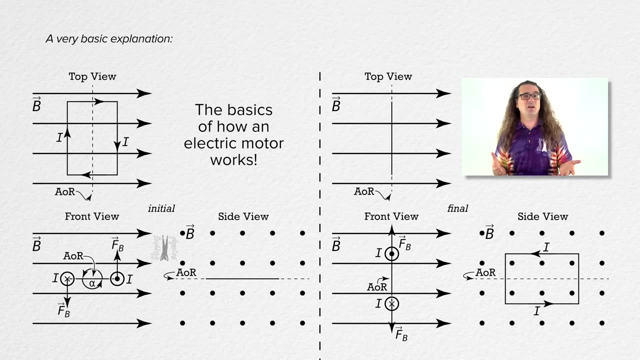 where would we ever see something like this? This is the basics of how an electric motor works. Eww Right, There is a lot more to how electric motors work, but I'm not going to go too deep. However, what we have shown here is the basic concept. Electrical energy is used to create. 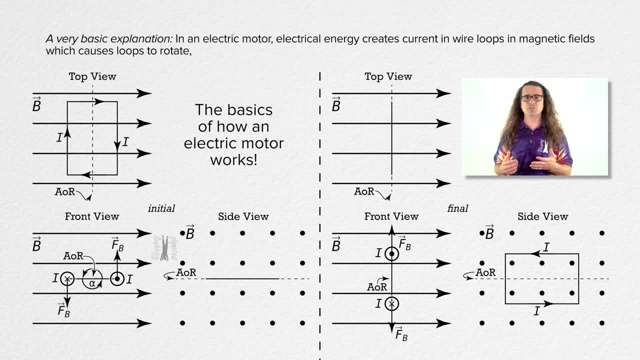 current in wire loops, in magnetic fields, and that causes the loops to rotate, effectively, converting electrical energy to mechanical energy to rotate things like engines. Sure, That seems pretty useful, Yep, But don't worry, there's more. Alright, Of course there is. Looking at the side. 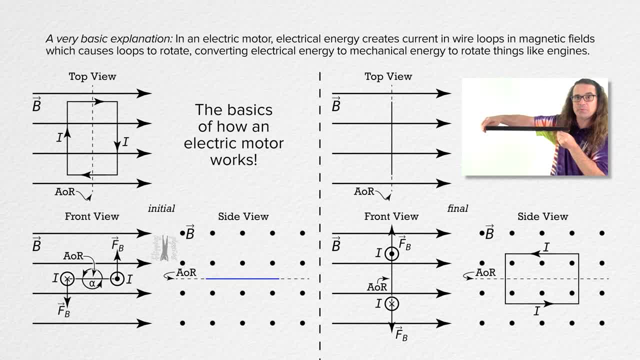 view realize. the current carrying loop goes from this position to this position while in a magnetic field. Can anyone tell me why I am pointing that out specifically? Again, in the side view, the current carrying loop goes from this position to this position while in a magnetic field. 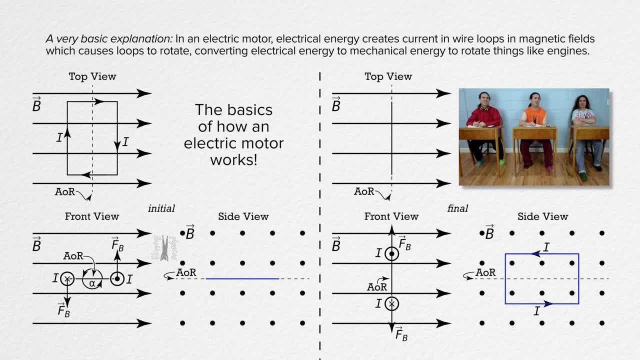 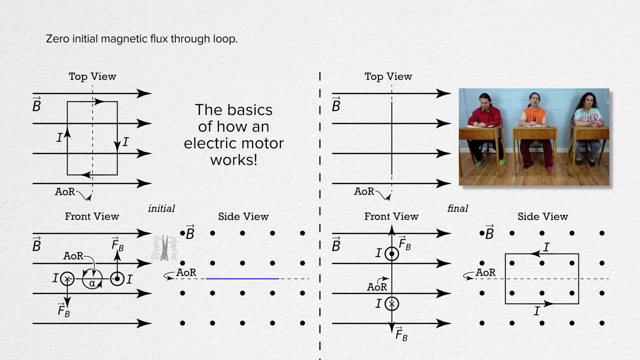 Ahhh, No, The magnetic flux through the loop increases from the initial to the final point. It does. Yeah, In the side view, in the initial position, you can see that there are zero magnetic field lines passing through the loop. Therefore, initially there is zero magnetic flux. 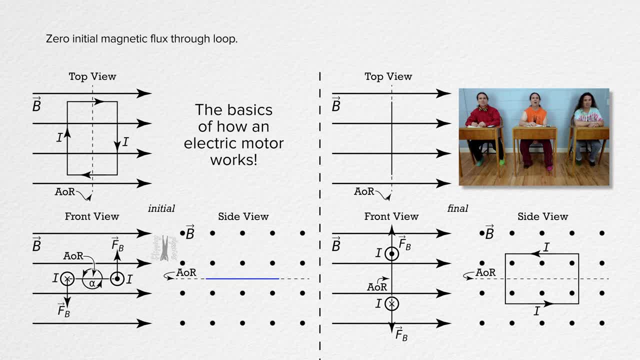 through the loop. After the loop has rotated 90 degrees, in the final position in the side view you can see there are magnetic field lines coming out of the screen and passing through the loop. That means that in the final position there is magnetic flux passing through the loop. 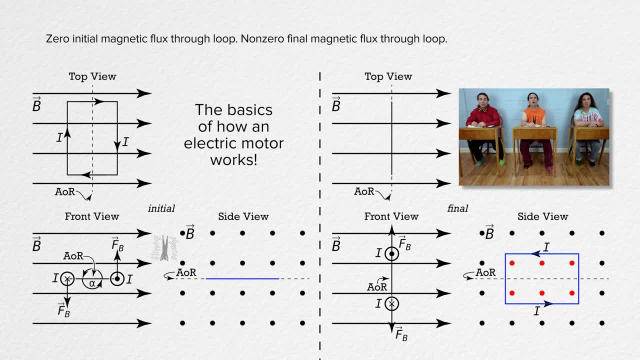 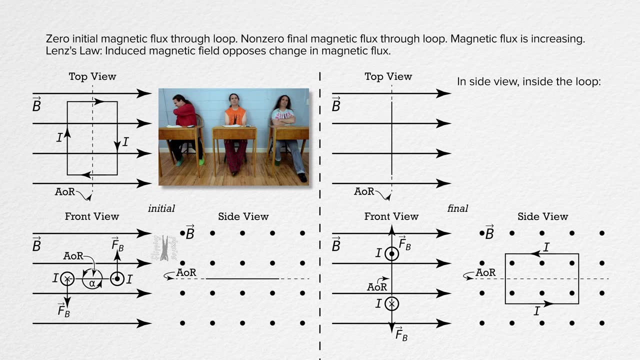 Therefore, from the initial to the final position of the loop, the magnetic flux is increasing. That means that according to Lenz's Law, there must be an induced magnetic field which opposes that change in magnetic flux Inside the loop. the induced magnetic field will be into the screen in. 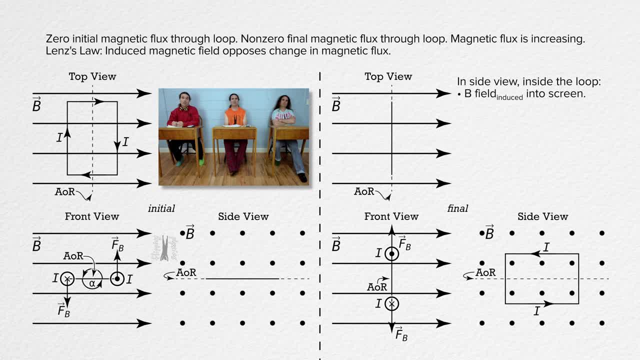 the side view again to oppose the increase in the magnetic flux And, using the alternate right hand rule, point fingers in the side view into the screen. in the side view into the screen inside the wire loop in the direction of the induced magnetic field. inside the wire loop. 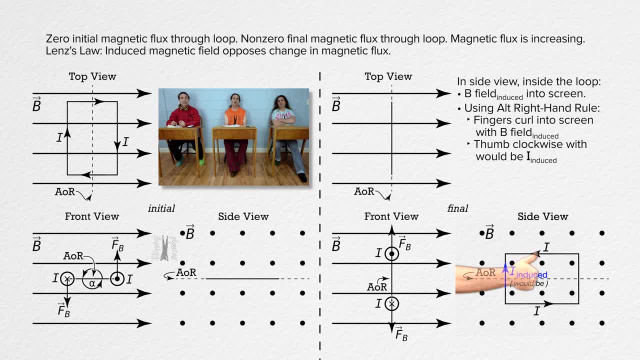 and the thumb points in the clockwise direction in the side view, in the direction of the induced current in the rectangular current carrying wire loop And that induced current in the wire loop which is clockwise in the final position in the side. 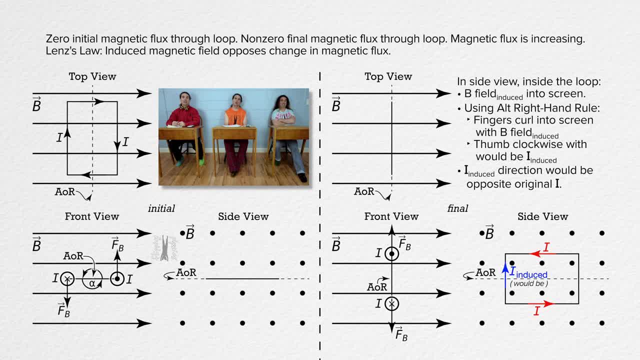 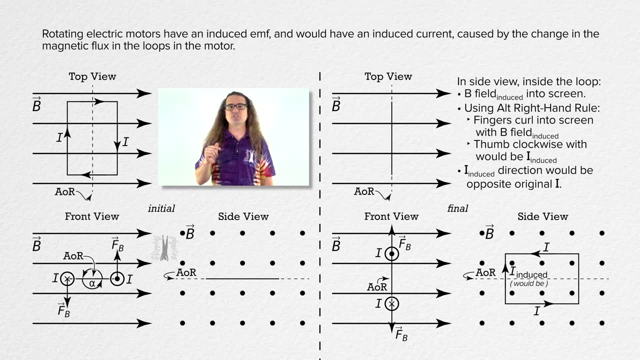 view is opposite the direction of the current. we placed on the wire loop in the first place to make it rotate in the magnetic field. Oh, Exactly, E electric motors. there is an induced EMF and there would be an induced current caused by the change in the magnetic flux in the loops of the motor. And that 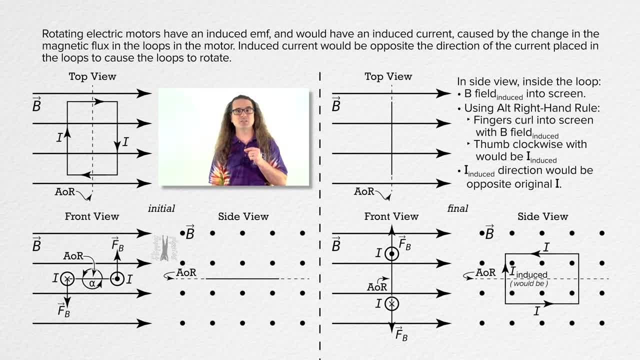 induced current would be opposite the direction of the current placed in the loops to cause the loops to rotate in the first place. Because this induced current would be opposite in direction from the current placed in the loops to cause the motor to turn in the first place, this decreases the current in the 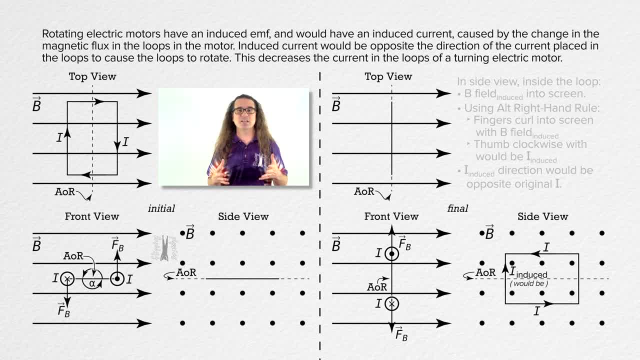 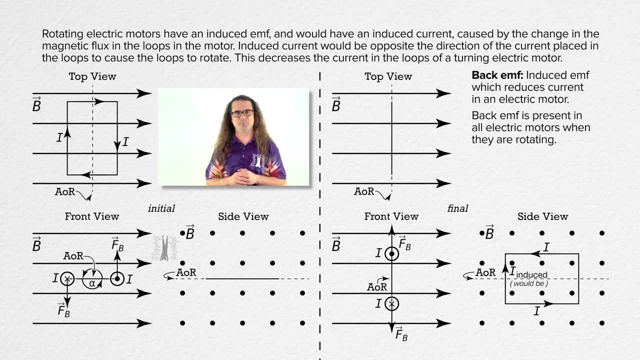 the loops of a turning electric motor. This concept is called back EMF, And back EMF is present in all electric motors when they are rotating. Realize this: back EMF is not present when the electric motor is not rotating and the back EMF is lower when the motor is rotating at. 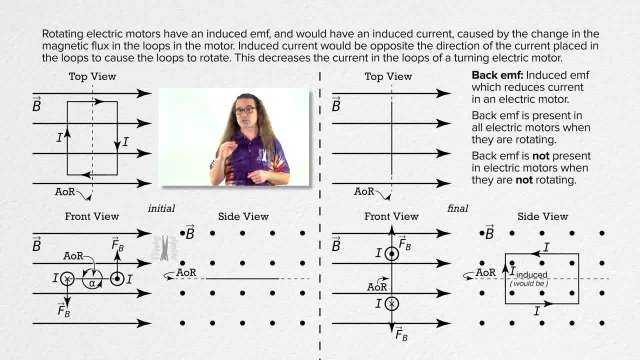 slower speeds. In other words, when an electric motor is first starting up, the current through the electric motor is larger than when the electric motor is turning at a constant angular velocity. This smaller back EMF, when an electric motor is just starting to rotate, can cause lights. 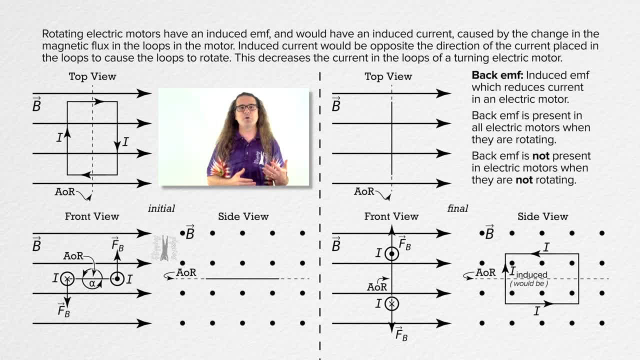 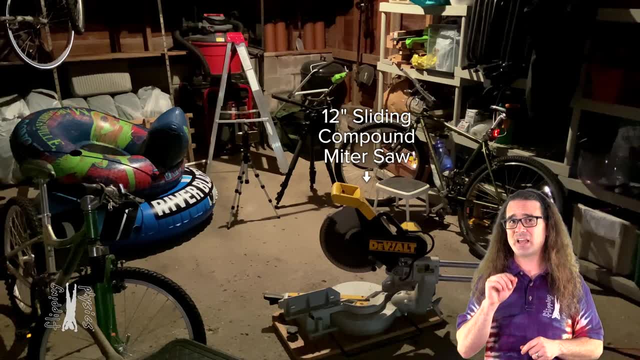 which are on the same circuit as the electric motor to dim when an electric motor is first starting up. You can see this occurs when I am standing in my garage using a 12-inch sliding compound. miter saw This garage only has this single light bulb to illuminate the space. 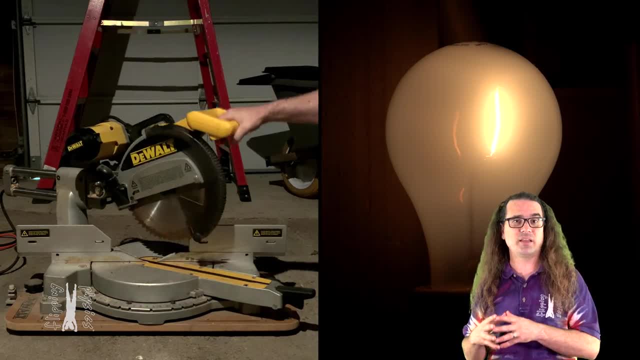 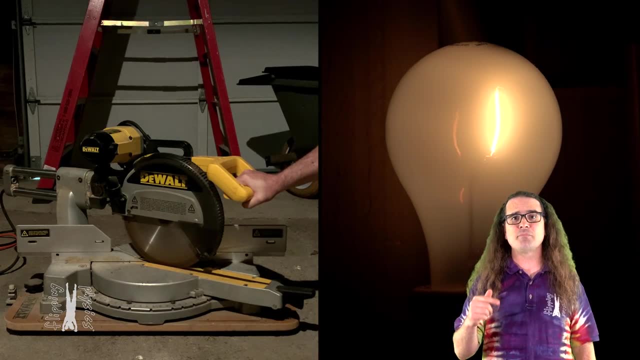 and that light bulb is on the same electric circuit as this electric saw. That means when I start the electric saw the lights dim because the electric motor in the electric saw at startup draws more current than it does when it is turning at a constant angular velocity. Again, notice the. 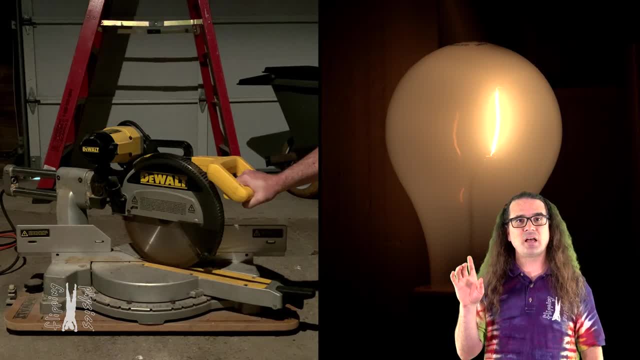 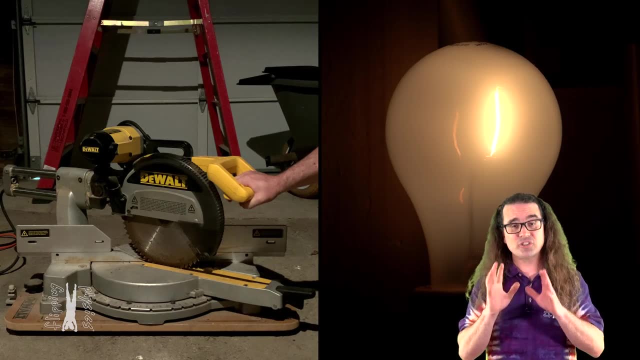 light. the light is at a normal brightness, while the angular velocity of the electric motor is constant. However, when I turn on the 12-inch sliding compound miter saw and the motor is just turning at a constant angular velocity, the electric motor is at a constant angular velocity. 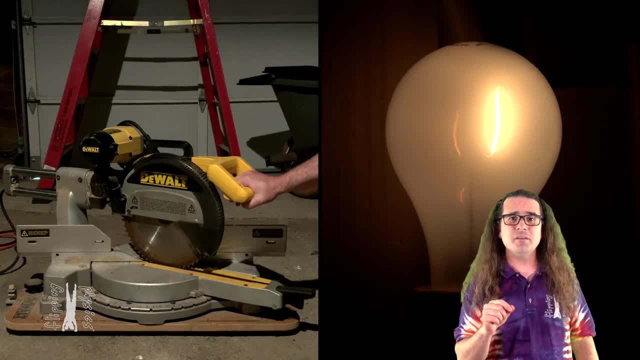 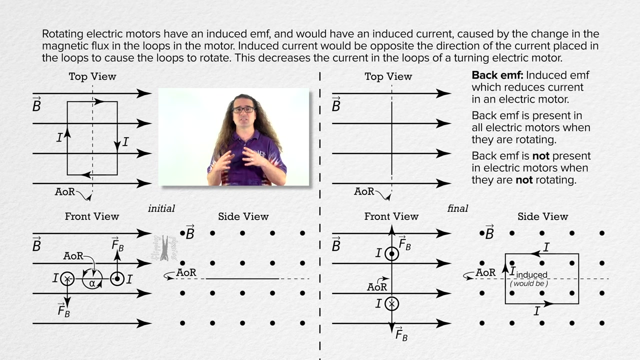 Even though the electric motor is just starting up, the lights dim because there is very little back EMF at the start. when the electric motor is just beginning to rotate, This decreased back EMF also happens if something suddenly binds the electric motor, causing it to stop rotating, which brings the back EMF down to zero suddenly and the current 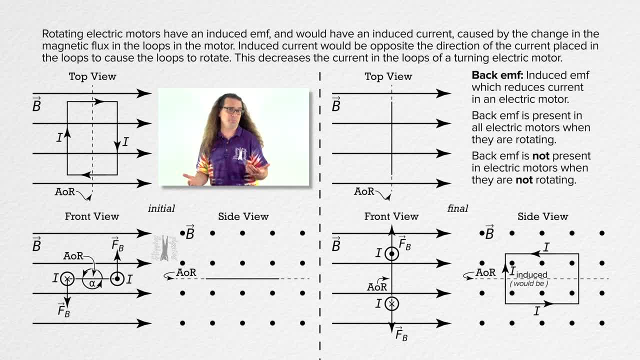 in the circuit increases suddenly and this can trip the circuit breaker because the current in the circuit is now above the maximum current. We will talk more about that in the next segment: current allowed through the circuit breaker. You've never done that, have you, Mr P? 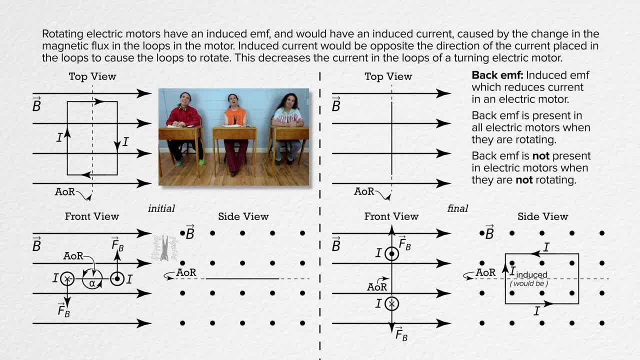 No, definitely not. I didn't think so. Why would the back EMF be constant when the motor is rotating at a constant angular velocity? Yeah, If a current carrying loop is rotating in a magnetic field like you showed us, then the back EMF should be increasing and decreasing as the magnetic flux through the 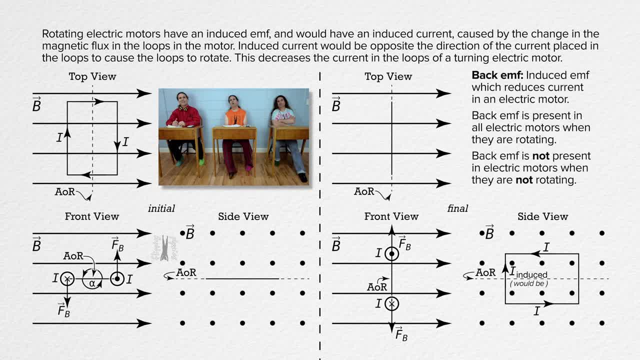 loop changes as it rotates in the magnetic field. Okay Well, I don't think it's worth getting into all the specifics about how a direct current electric motor works. I guess what I'll say is that it includes a very large number of loops. 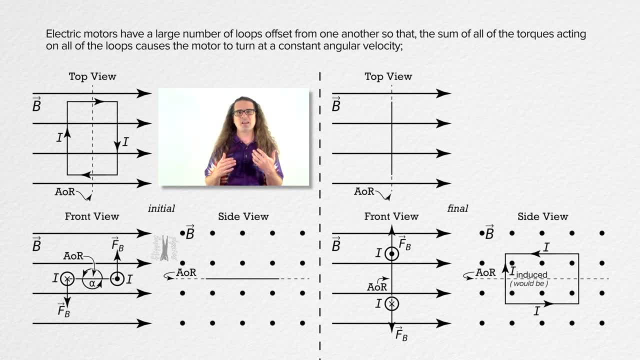 which are offset from one another, to make it so that when you add up all the torques acting on all of the loops, the motor turns at a constant angular velocity and therefore the back EMF has a constant value. It also includes something called a split ring commutator. 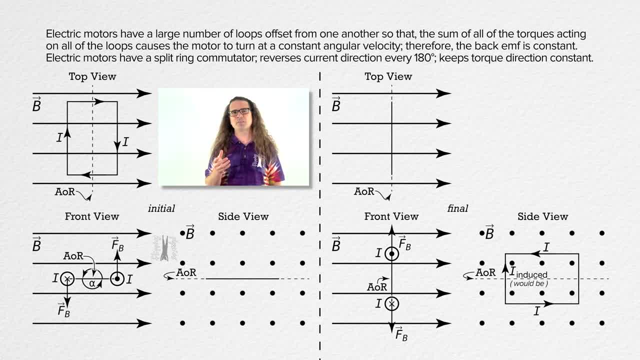 which reverses the current every 180 degrees, keeping the torque on each loop in the same direction. Ah, Sure, Yeah. That concludes my review of induced forces for AP Physics C- Electricity and Magnetism. Next time we are going to review inductance. 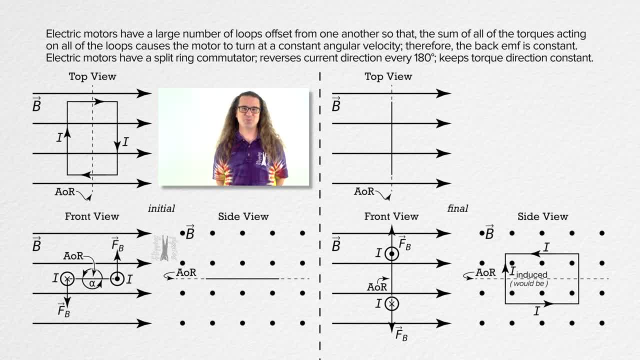 Thank you very much for learning with me today. I enjoy learning with you.